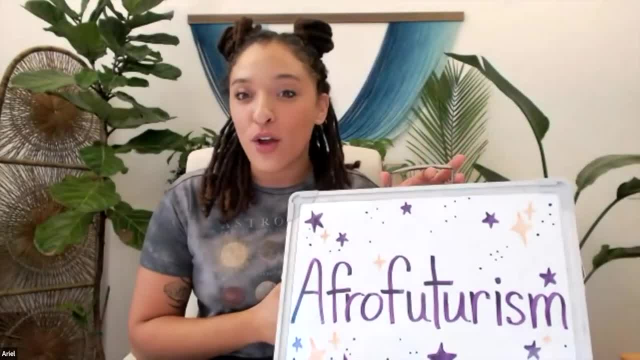 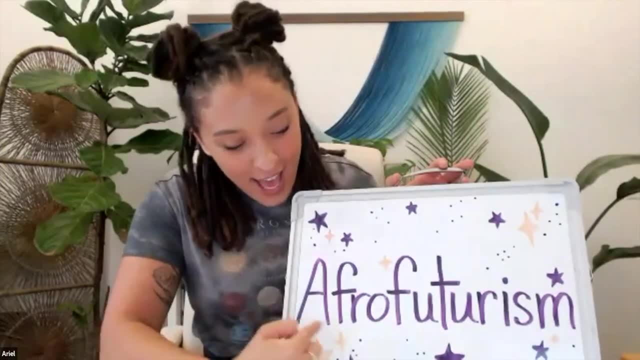 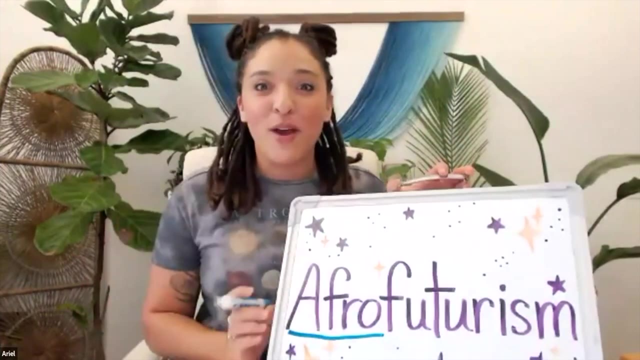 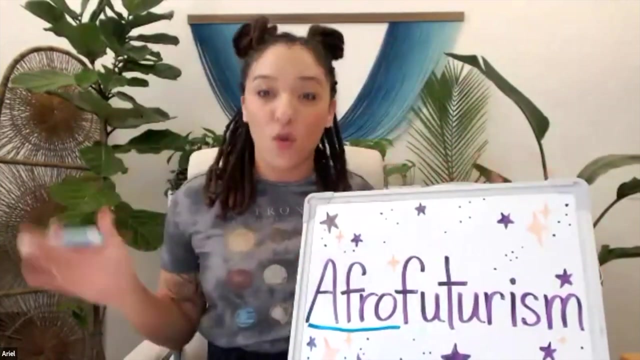 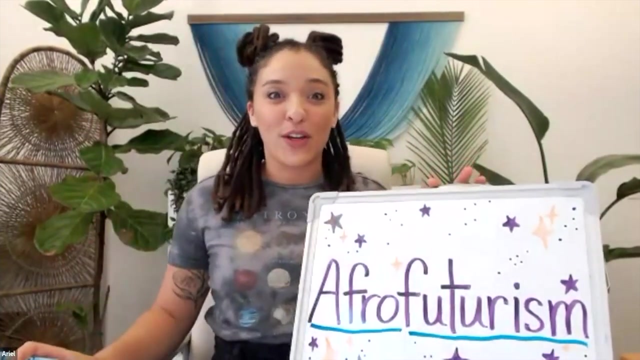 like that word means Afrofuturism. The Afro- let me make sure I write that in for you. The Afro part of the word is talking about Africans, African Americans and people of African descent from all over the world. Futurism sounds like the word future. 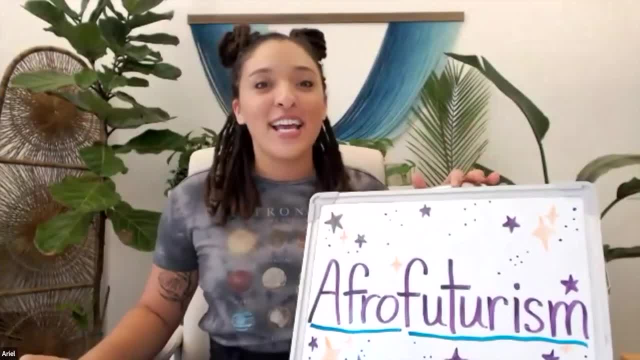 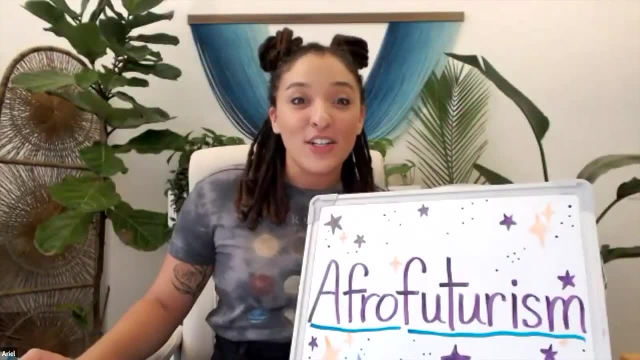 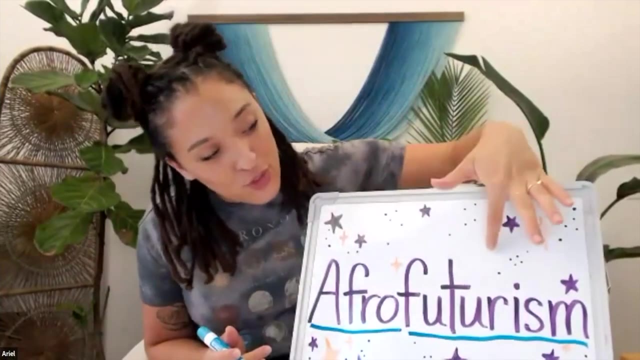 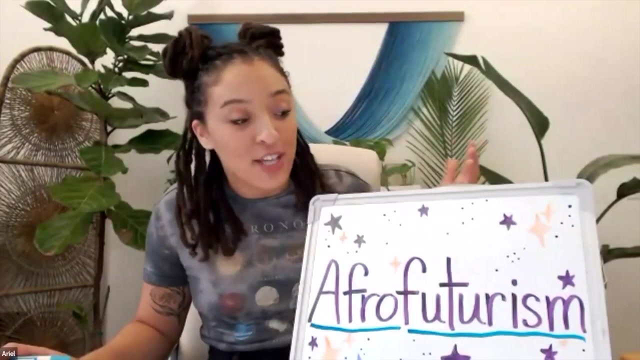 Excuse me, The future is what we haven't done or haven't even seen yet. Tomorrow is the future, Next year is the future. Thousands and thousands of years away is the future. Afrofuturism is what people of African descent imagine the future can be, And they may show their imagination. 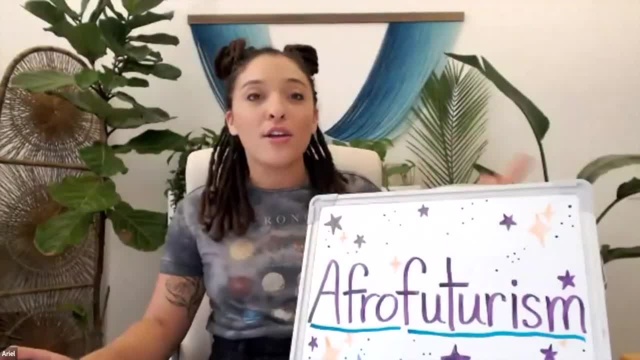 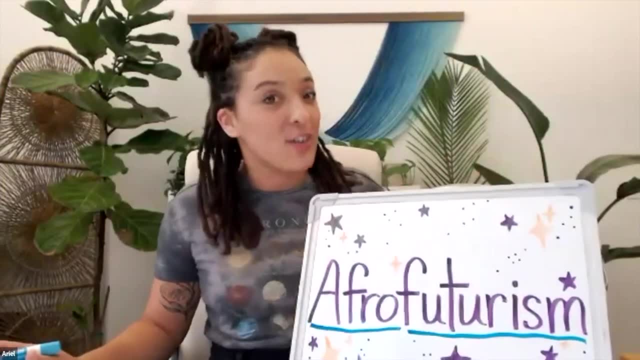 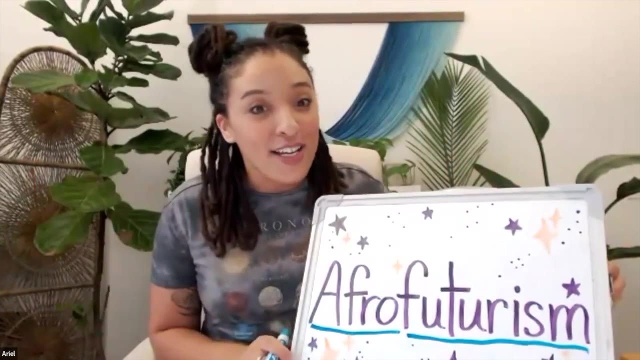 and their hopes for the future through art, music, stories, movies and more. Sometimes the future is here on planet Earth, and sometimes that future is in space or a whole new world that doesn't even exist yet. The artist we are talking about today. 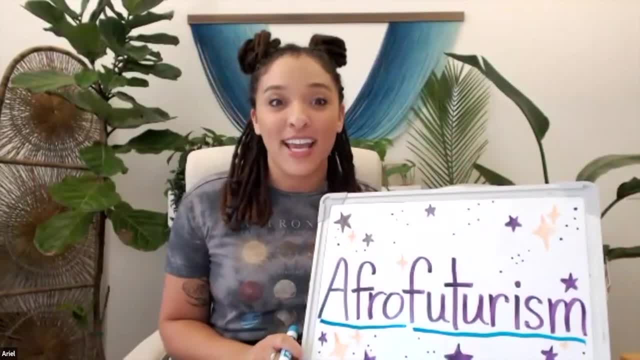 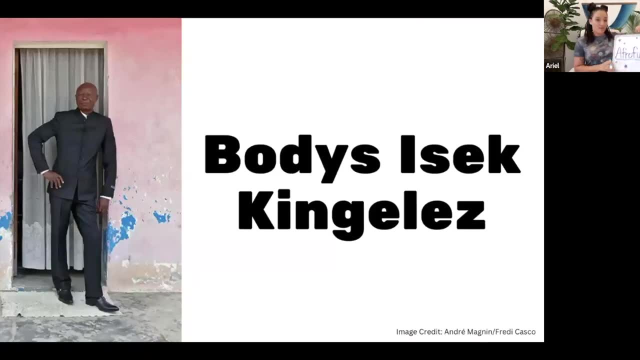 had a vision for what our future buildings can look like on this planet one day in the future. Let's jump in and learn about BOTUS Ezek King-Velez. King-Velez was an artist from an African country called the Democratic Republic of the Congo. 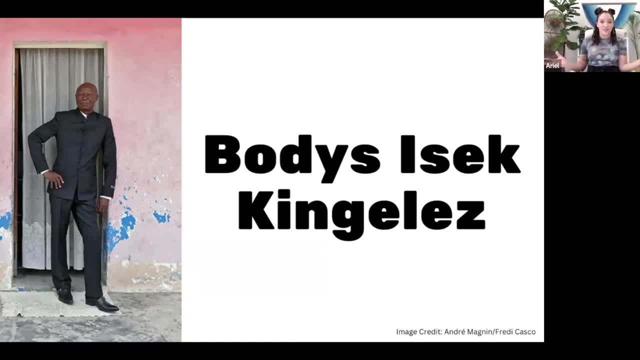 And he grew up in a small village with a really big family And ever since he was a child he wanted to change the world. He wanted to help people and he wanted to make the world a better place. And when he grew up he found a couple ways that he could do that. He was a teacher. We know that teachers are amazing health professionals. 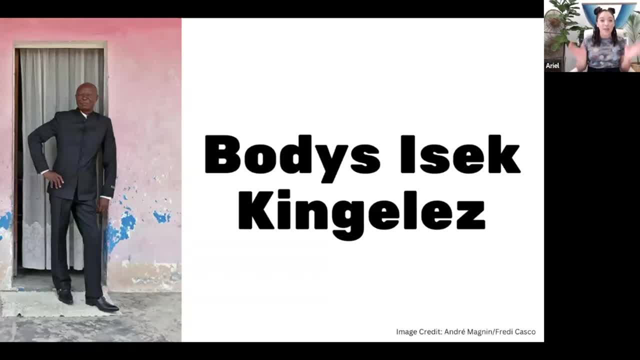 He was a teacher. We know that teachers are amazing health professionals. He was a teacher. We know that teachers are amazing health professionals. I'm sure some of you have teachers with you right now on the other side of the screen. They help our world become a better, more beautiful place by teaching children about new things and helping students like you learn skills that you can use to change the world in your own different and amazing ways. 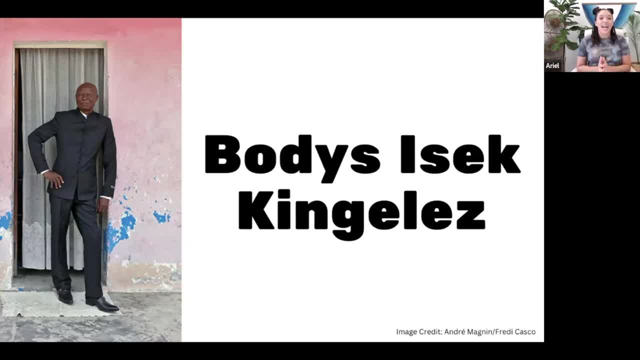 Thank you, teachers. He also worked at a museum to help make sure that his country's history was shared with people, And that's the way I also like to help the world. But one day he discovered that his favorite way to help the world was using his imagination. 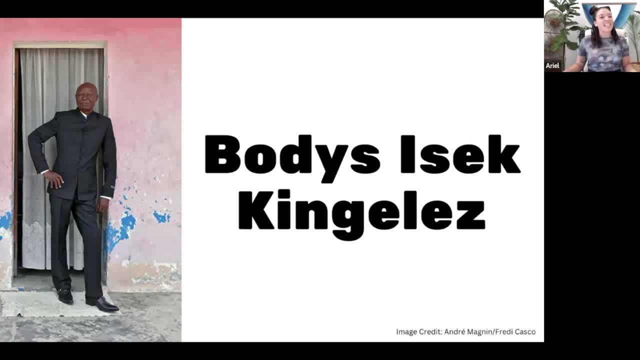 Now, what is an imagination? It's kind of hard to describe because it's not something we can always touch or feel or see. Imaginations are pictures and ideas and things that we might see inside. We might see things inside of our heads that aren't fully real right now, but they are real to us in our heads and in our hearts. 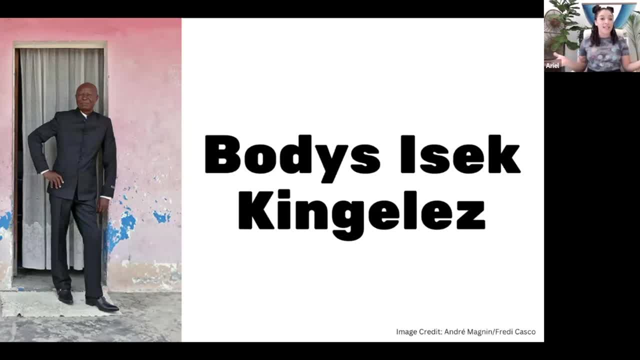 We might use our imagination to create a picture in our mind. We might use our imagination to play pretend with our friends. We may use our imagination to create anything we don't have right now but want to have one day, like in the future. 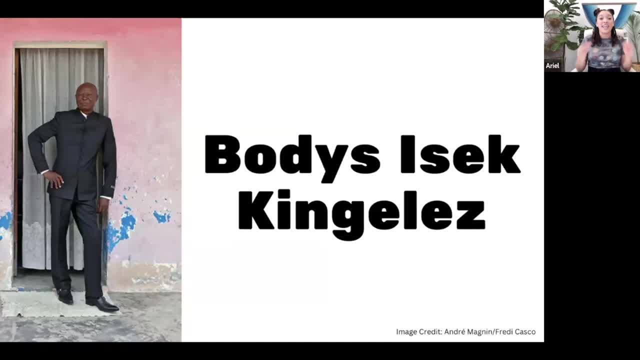 Our imaginations can create the future. Kingel has wanted to help other people by using his imagination. but how can an imagination help other people if it's inside your own head? Hmm, well, Kingel has said that it was really important to him to build an example of what you are imagining inside of you, so that other people can see it too. 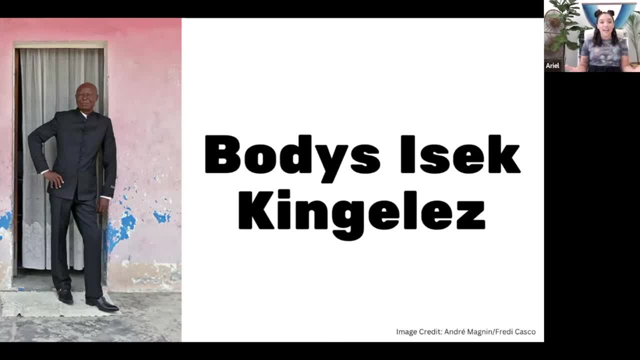 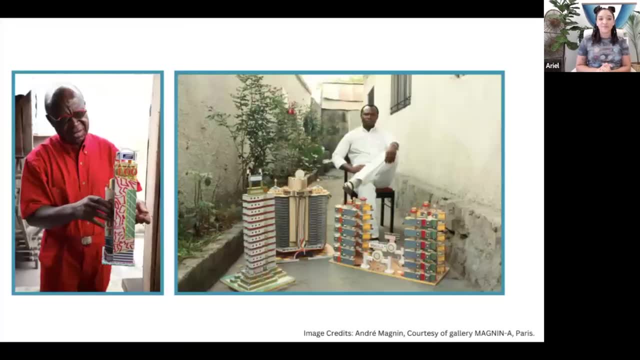 And maybe when they see it, you can work together to make your imagination come true. And that's why he started making his art. What kind of art did Kingel make? What do you keep seeing in these pictures? In one picture, he's sitting outside of his home with his art. in another picture, he's holding it to show to the camera. 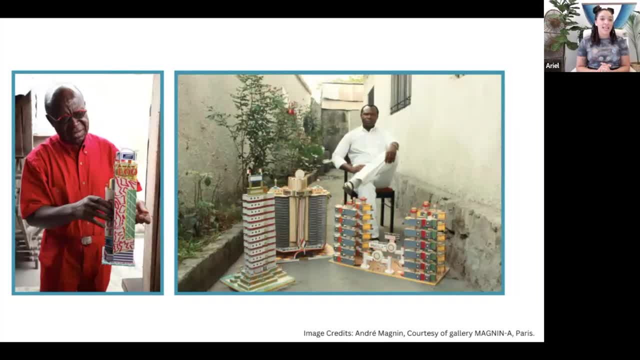 In another picture he is holding it to show to the camera. In the live video, Kingel is walking in his room with his imagination. In one picture he is sitting outside his home with his imagination. In another picture he is holding it to show to the camera. 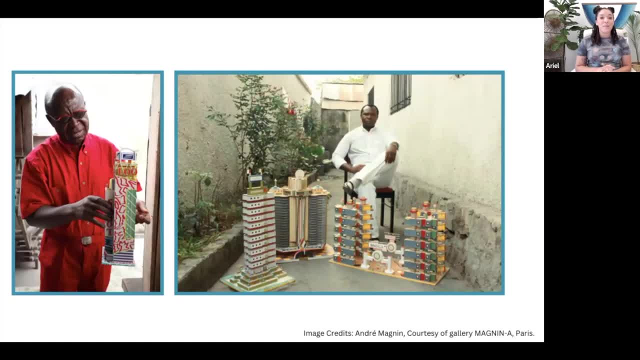 made many buildings. King Gilles imagined the small towns and the big cities in his country and from countries all over the world looking a lot differently than they did back then and that they do right now, When he imagined a city where people live in peace, where they all get along. 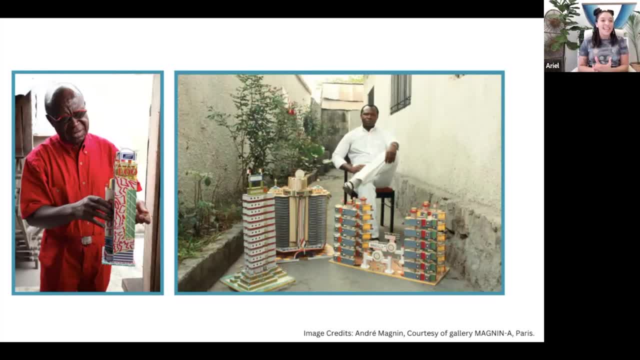 and are healthy and are surrounded by beauty. he saw buildings of all different shapes and colors, with different kinds of windows and doors and details than anyone else had seen before. King Gilles imagined and created over 300 different buildings and I want to show you how creative he let his imagination get. Before I show you, can you imagine or picture in your mind? 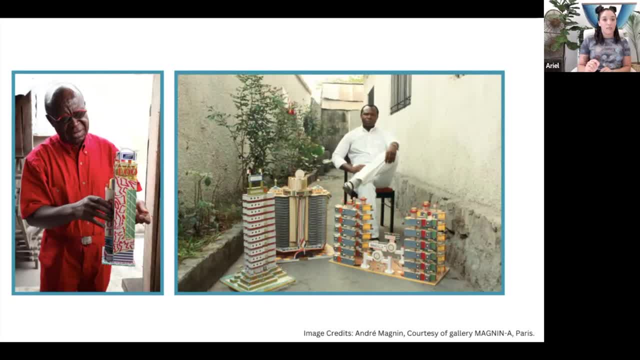 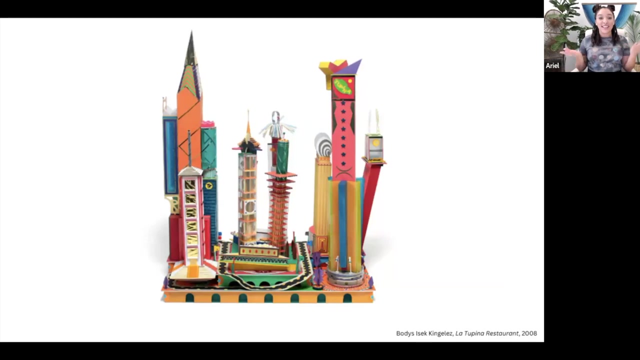 a restaurant or a place you get food from. Picture it in your mind. And now that you have that picture, did it look anything like this? In King Gilles' imagination, a restaurant in the future looks like this: What do you notice about this restaurant? Is anything about it the same as the one you? 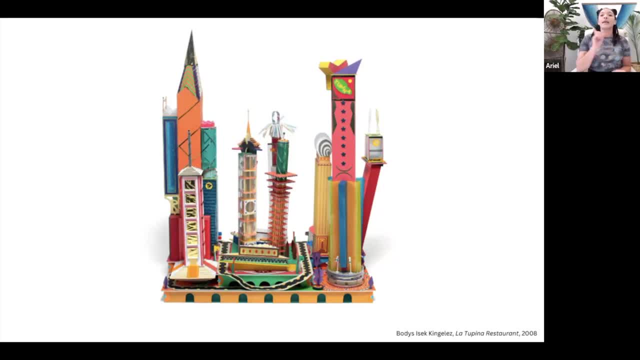 pictured in your mind What's the same and what's different. You can share your thoughts in the chat, Share with us in the chat your ideas, or you can talk to someone who's with you on your side of the screen today, While we wait for some friends to share, I'm going to take a close look and think about what. 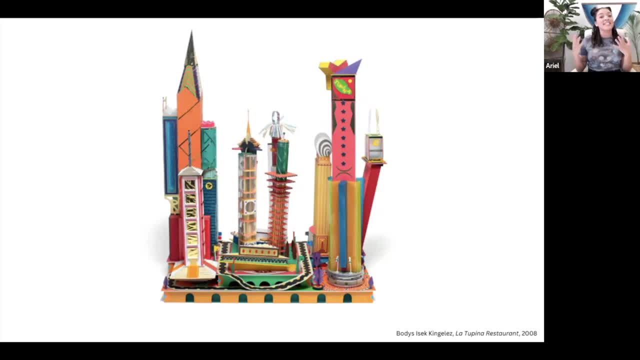 restaurant I was picturing And it did not look like this. The picture that the restaurant I was picturing is usually like a beige or brown color on the outside and something I was picturing is a lot of different colors. I'm seeing orange and blue and green. Some students are saying it looked 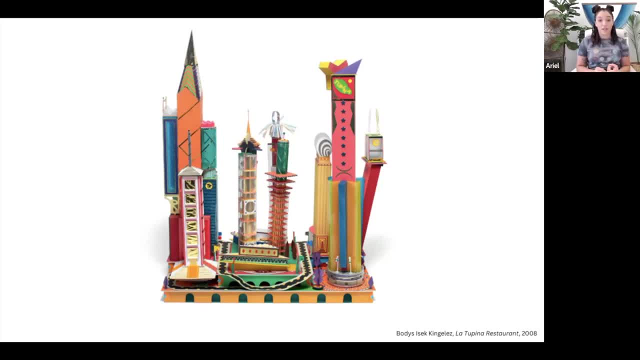 a lot different than any of the restaurants they were picturing. I see also some pink and red on this restaurant And I'm really excited because I love pink and there's usually not pink restaurants out there. I'm also noticing some different kinds of shapes than I would see with a restaurant. 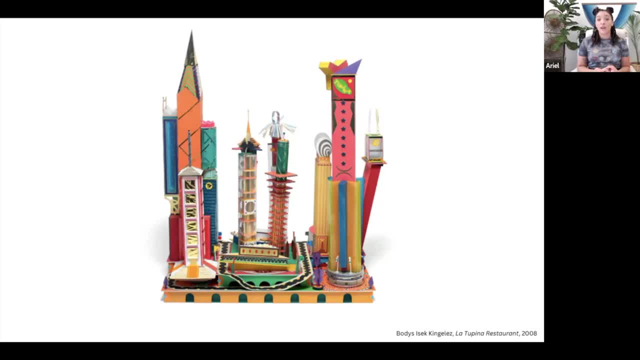 Someone shared that this restaurant is very colorful and it looks like there's buildings inside of a building and then also a road and railroad tracks and multiple buildings. So I'd be curious: which part do you eat in, Or is it? are there just? 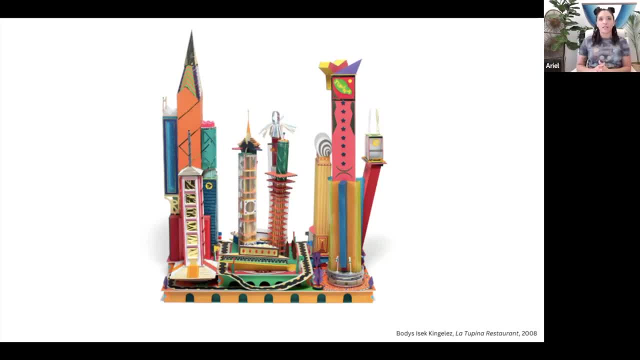 places to eat in each of those different parts. Some other friends noticed that there's different colors and this restaurant seems really big and there also seems to be some water. I was noticing that as well. Now, one thing that I'm noticing also is all of those different towers. Can you count? 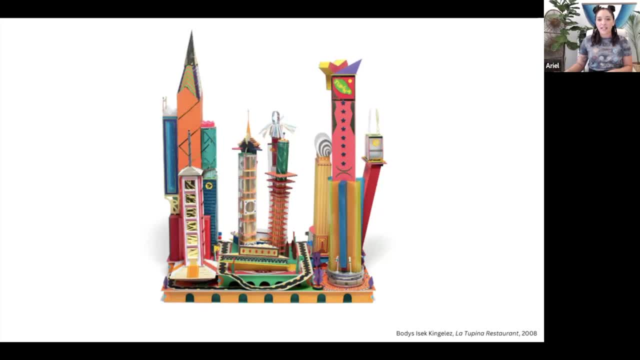 how many towers there are. It's a little bit hard to tell if some are attached or if they're not in their one tower or their multiple towers. Let's try and count together. I see one, two, three, four, five, six, seven, eight, nine. 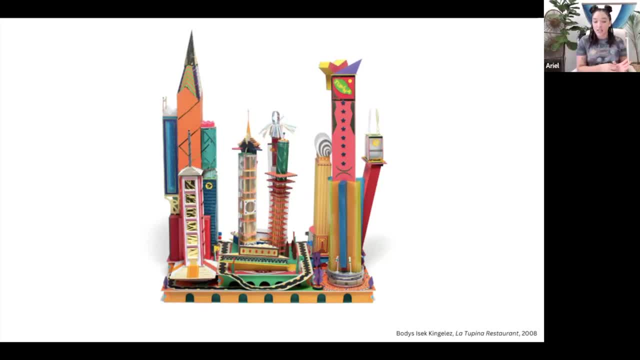 There might even be more if we were able to turn it around and see the other side, but there's nine towers on this restaurant. Oh, another student noticed some water flow. I feel like that's probably a really pretty view to look at while you're eating. 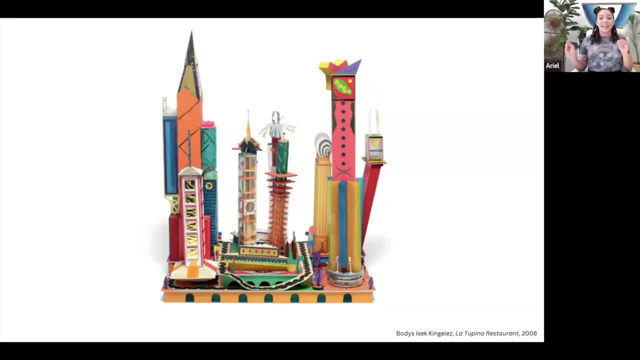 But wow, what a restaurant, And I couldn't have imagined this just yet. That's not what I would have imagined in my brain of a restaurant, but that's what Kinglaz saw. What about this building? Let's take a look at another building. 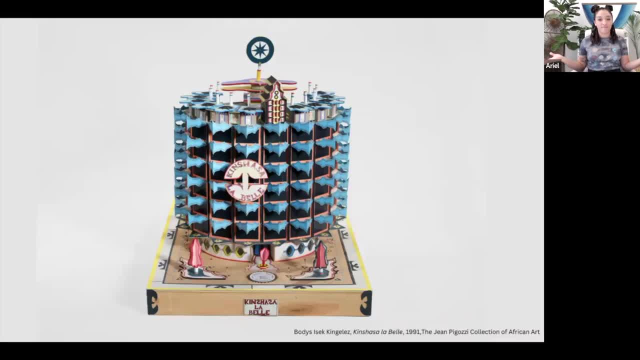 What kind of building could this be, Any ideas? It's like round. It's probably really tall in real life. Ooh, someone guessed a hotel, And you know what. To that class. that is actually correct. So I wonder your imagination is working a lot. 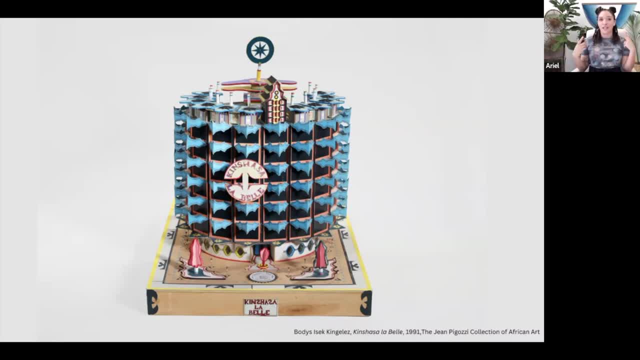 like Kinglaz's. This was a hotel in Kinglaz's imagination. I would not have guessed it, but someone else. they were on the same page as Kinglaz. Oh, another class at a hotel too. Oh my goodness. 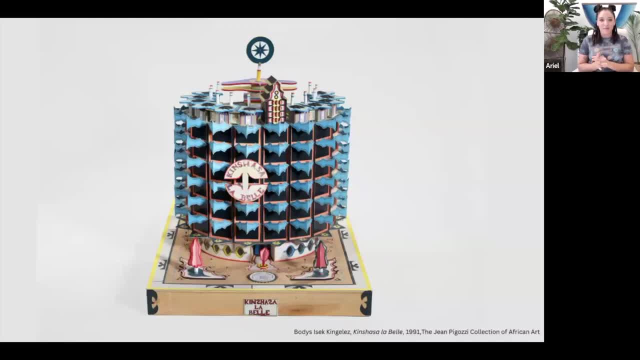 That means our imaginations are really working today, But one of the things I love about imaginations and the future is that they can be different than anything we've seen before And, at the same time, they can still be something that we know or that we really like. 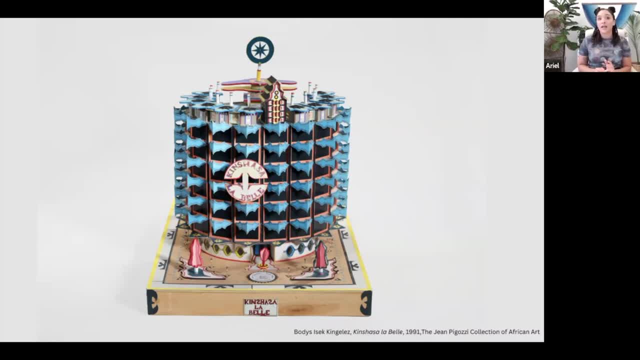 Someone's noticing that this building looks a lot like the Renssen. I think this is the Renssen building in Detroit. I have not seen that building. I'm going to have to look it up Now in his imagination for this hotel. 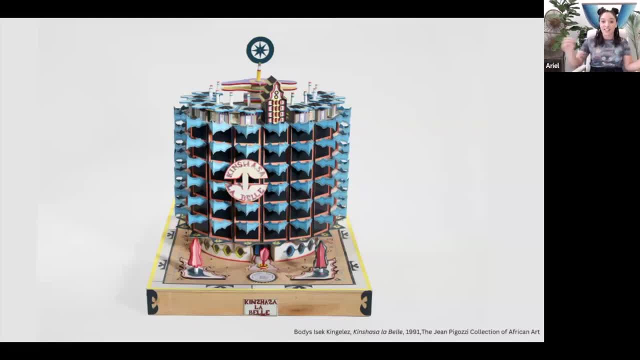 Kinglaz saw big blue butterflies surrounding it, And that's what he tried to create here. I think he did a really great job of showing what butterflies would look like if they were all around a building. Behind each of the butterflies would be a balcony where people 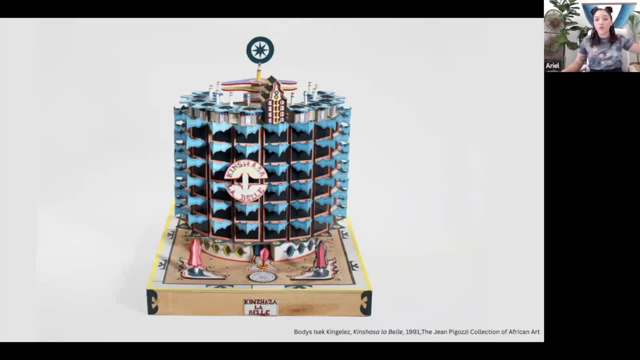 could stand outside and you could like look at the view from your hotel room. Now I'm wondering for all of my friends out there who are already using their imagination: if you could decorate a building with an animal or an insect, what would you choose? 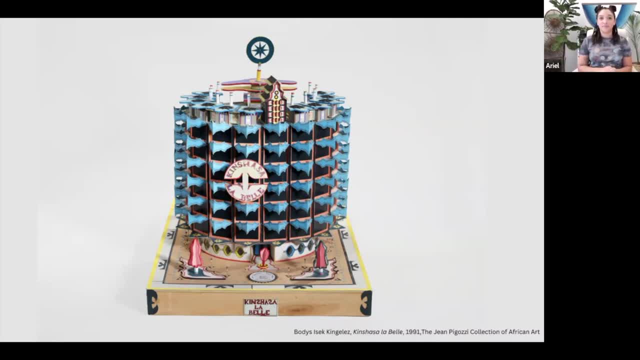 I already know my idea. Ooh, someone would like to see a building with a fox on it. Now, this could be a fox like what I'm used to, which is like a red or reddish orange kind of fox, but there's also some white foxes, some black foxes. 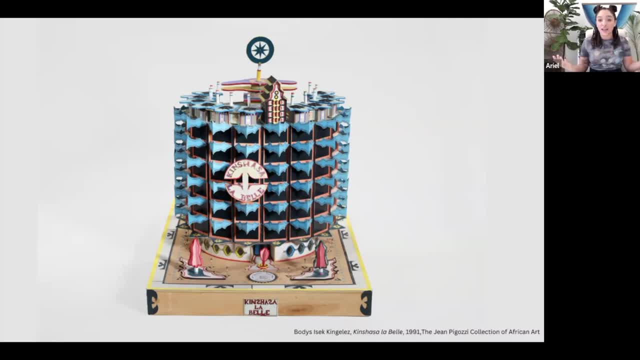 Ooh, someone would like to cover a building with whales or an elephant lions. Oh, these sound like they'd look so cool. We have some friends would want to use a cat, a snake, a shark, a mouse or mice, bison, wolves, a cheetah. 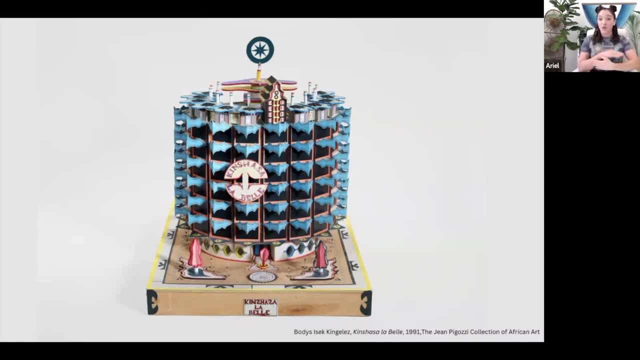 Now a cheetah, since it has that special pattern all over it. that could be a really cool thing to see around the whole building And someone was noticing they really can tell that those were butterflies. They'd also someone said they'd like to see a building. 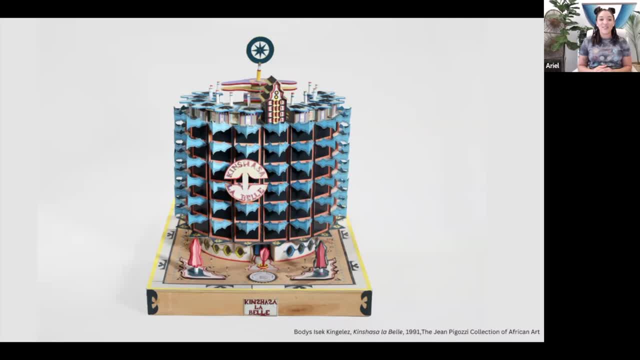 that looks that has some chinchillas on it. Ooh, what you know, what would be so cool Is if the building also felt like a chinchilla, like so soft on the outside, instead of like bricks or something like that, you know. 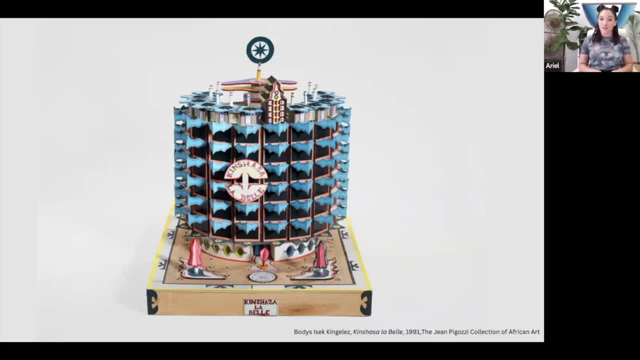 I'd be a little bit unusual, but that's what our imaginations and the future can be, anything that we think of. right, There could be horses that are going all around, A snake, a shark, bats and bobcats. So far I don't think anyone has said you know, I thought I'm trying to figure this out. Yeah, I don't think anyone has said: you know, I think this was just a bad idea. There's no way you can figure this out. There's no way you can figure this out. There's no way you can figure this out. 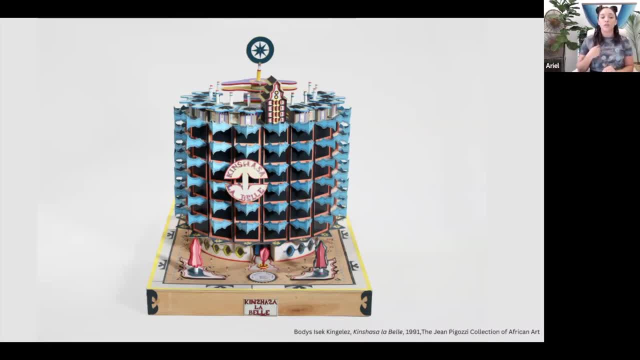 Uh-huh, And an idea I also had, which was I would love to see some birds around and maybe they could be hanging and kind of they could move with the wind around the building, Or what if there was some fish? Someone did say whales, but there could be whales and fish all around. 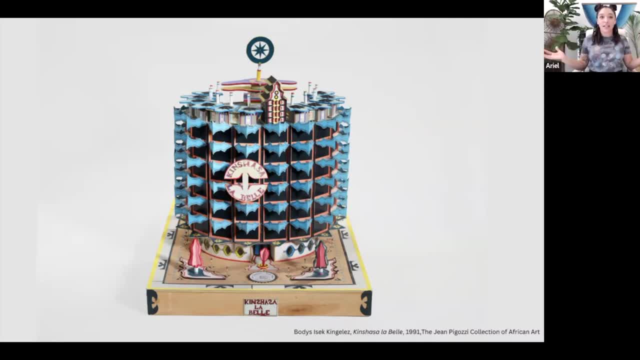 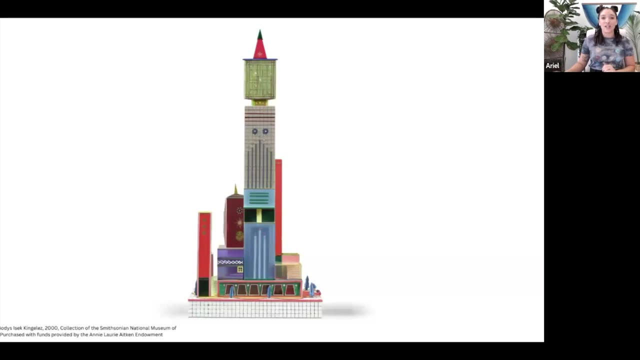 A dragon, an octopus. Oh my goodness. These are all really cool ideas. Thanks for sharing everyone. Let's take a look at one more building. One more building For now. This building is in the collection at the National Museum of African Art. 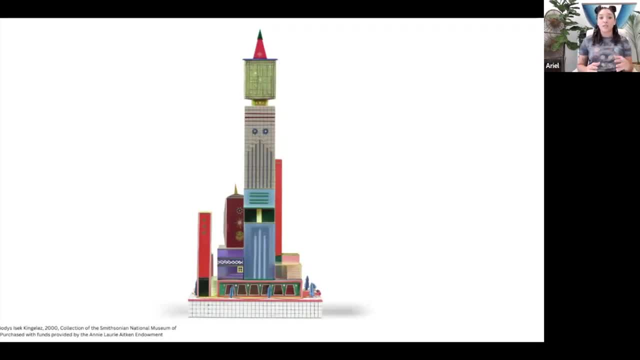 And I was thinking that, since Kingelez imagined that this would be a real building one day in the future, we should look at it like it's a real building and use our close looking skills to figure out how an architect or an engineer or a construction worker 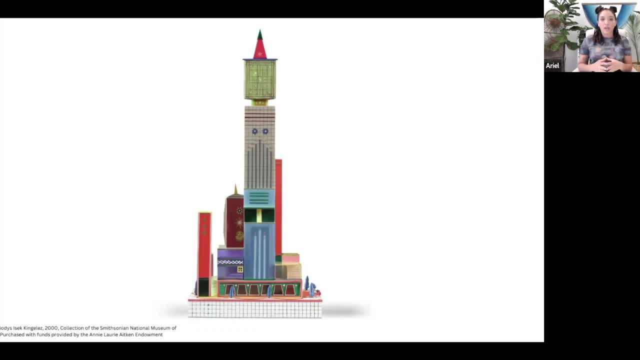 put This building together. You think you could try that with me. We can try that, All right. So now I have a tool for us to use. It's from our friends at the National Building Museum And it's something that you can use in your actual neighborhoods too, So later you might take a walk around and look at some of the buildings in your neighborhood or around your school. 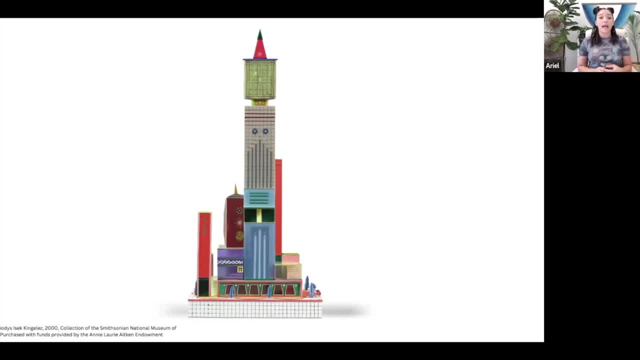 We are sharing it with you in the chat now, but I'm going to guide us through just two parts of it. The tool is: The tool is like a checklist that shows you all the different kinds of things you want to think about when you are looking at the buildings around you, in your neighborhood or for us today in Kingelez's imaginary world. 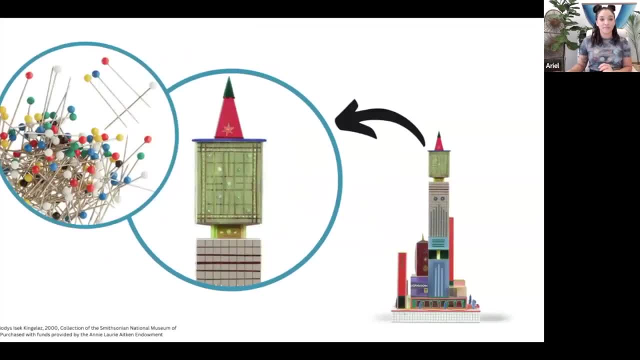 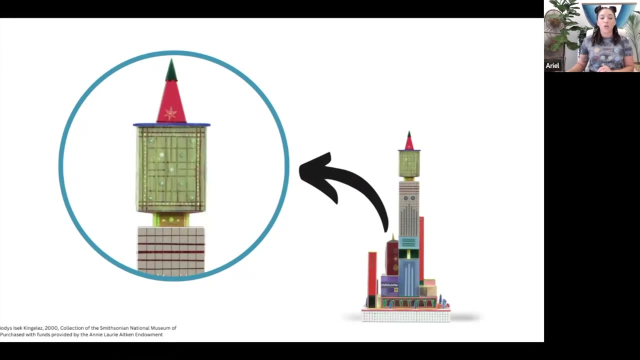 So let's get started. Oh, let's see One second. Let's go back. one slide there. There we go, All right. So one of the things we want to think about when, When we're looking at a building, is: what is it made out of? 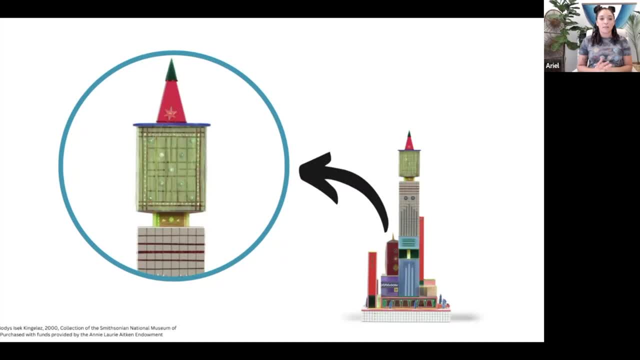 Now, what do you? what are some of the things that you think that King glass might have used to make his art? Since these were small buildings and not big buildings, He didn't need to use things like wood or bricks or concrete. So someone said that he probably use some cardboard. 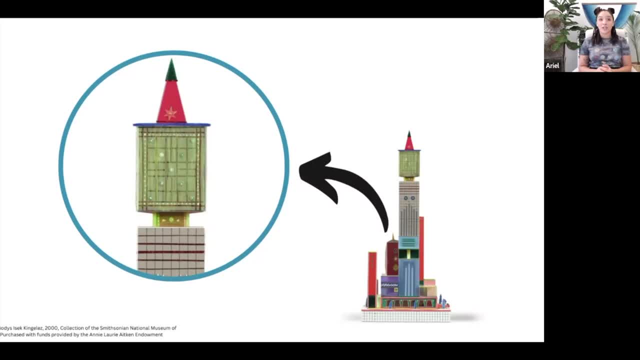 That's true. He use some cardboard. He use regular. He use regular paper that he had at his house pieces of plastic- and that's true as well. he used plastic that was from recycled materials like things like that might have some food in it at some point, but you take the food out and use it to make a building instead. even though King glass made these really extraordinary pieces, he used really ordinary materials. his mini buildings were made with regular things like paper and scissors and things like that. 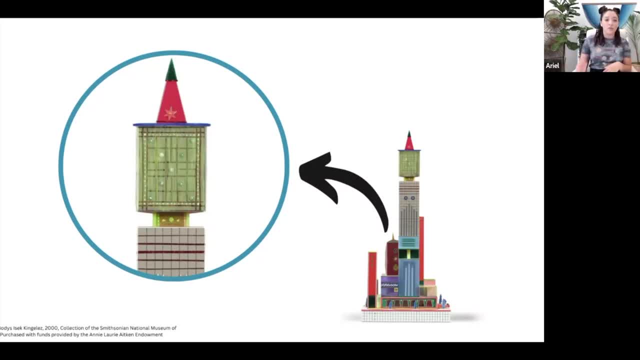 things like paper and scissors and things like that, things like paper and scissors and things like that, and glue and recycled materials and foil and bottles and boxes, things like that. Someone mentioned he could have used wooden blocks. So yeah, he might have like stacked some blocks on top of each other to make his buildings. 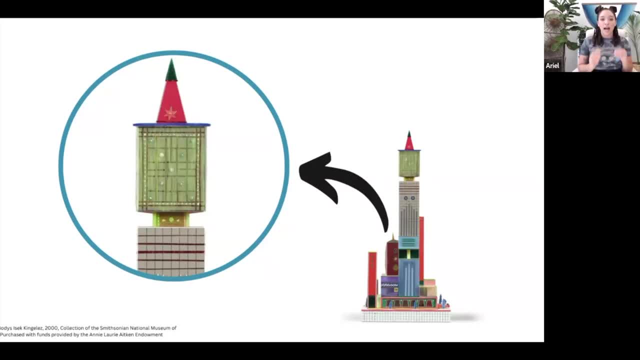 When we zoom in at the very top of this building, What do we see? what did he use to make this part of the building? I see, Hmm, I see some lines and I see I see some dots, And those dots are looking like 3D to me, not just markers or paint painted on, but 3D, something that is lifted off of the building. 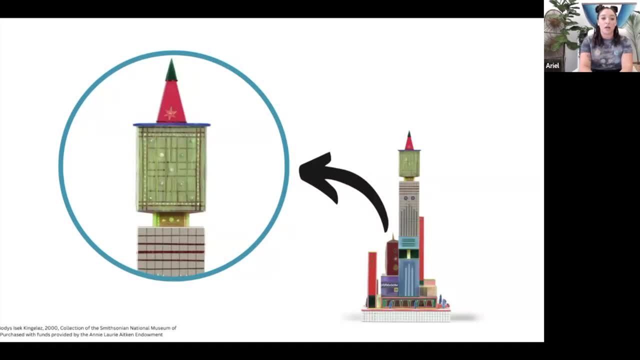 Now we got a little bit of a sneak peek, but what do you think those dots could be made out of? what material did he use to build that part of the building? Someone said it looks like pearls. Now, that is, that is Now. that is, that is. 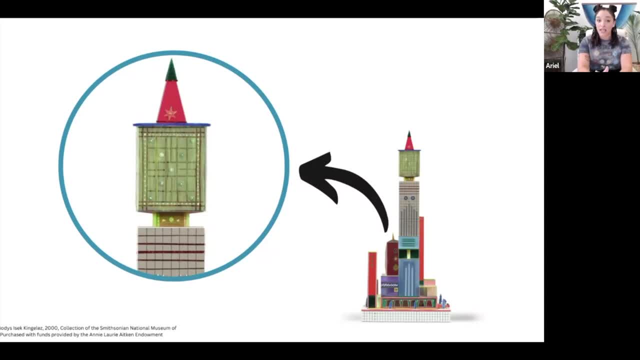 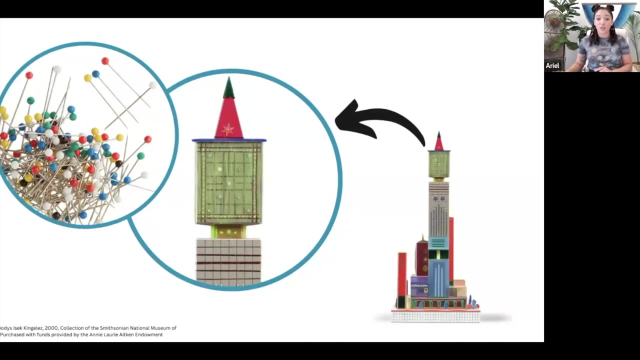 This is a really great idea. they look kind of round and shiny. Someone guessed that it could be push pins. Let's find out. Huh, they were pinned. someone guess bees, which is another really great suggestion. and marbles, beads and marbles. they're thinking of things that are round and small that you could glue on or add on to the building. 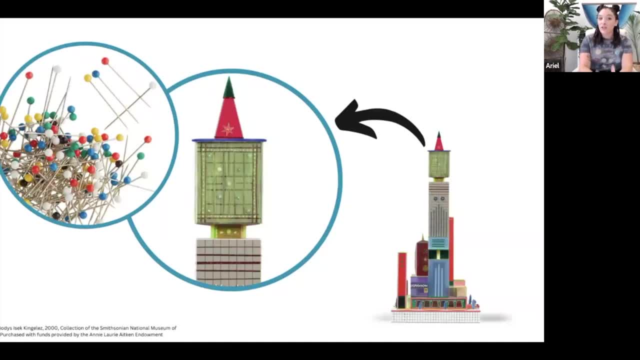 Now, have you seen kinds of pins before? Now, have you seen kinds of pins before? for They're usually used to hold fabric together when people are sewing, And sometimes people use these to put things on a bulletin board, like pieces of paper on a bulletin board Sometimes. 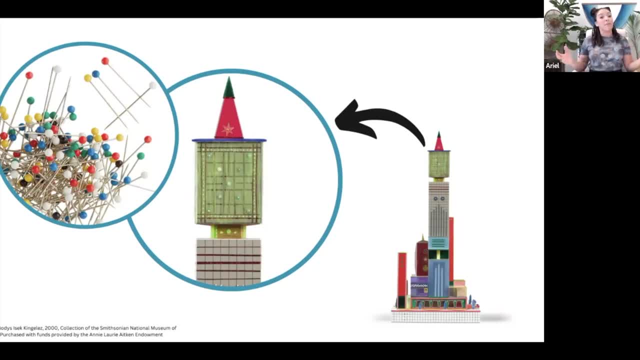 people use these kinds of pins to mark a map and show different locations on the map. I think it's really creative of Kingles to use something like this for his buildings, And some people even thought of some other materials he could use, like rubber bands, Play-Doh, green cotton. 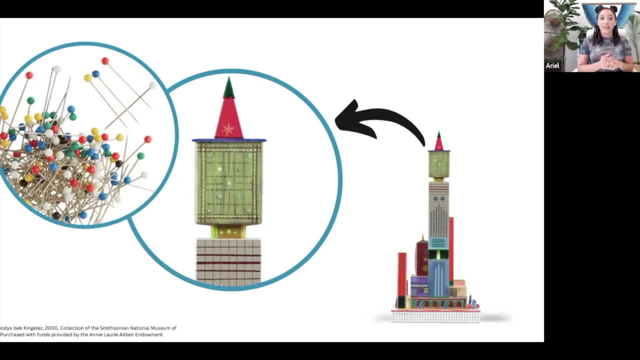 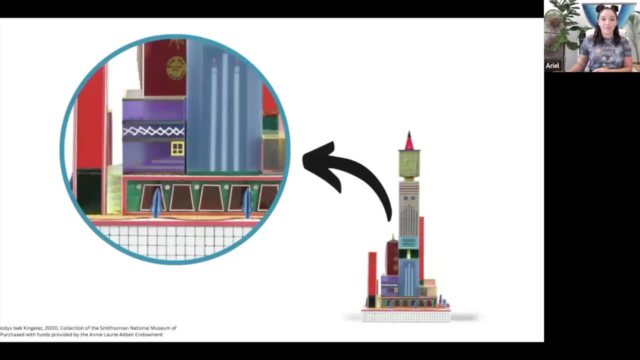 real blocks, toothpicks. These are all really great ideas. Let's look at one more part of this building. Another thing we want to look at when we are investigating a building are the shapes that are used, especially the different shapes of doors and windows. 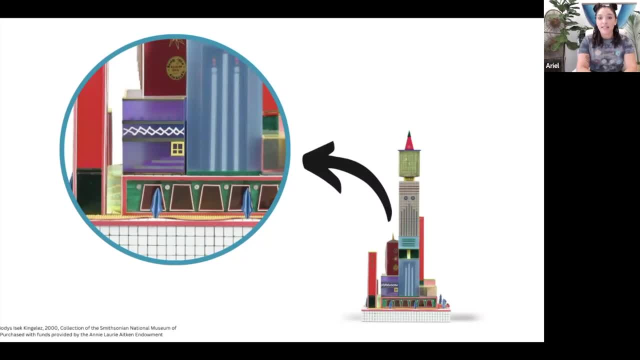 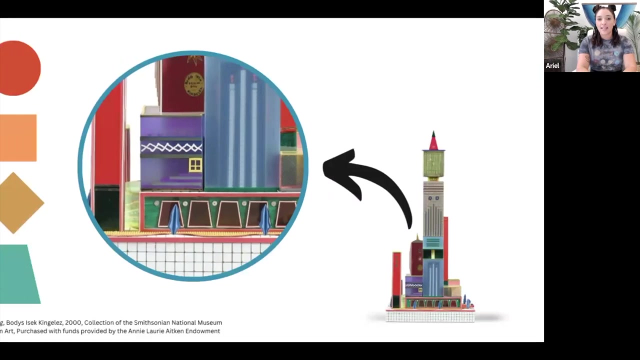 So if you look closely at this part of the building, what shapes do you see? Someone sees a square, And let's see, I also see a square. It's like a tiny yellow window. It's one square and then it has four little squares inside of it. Someone's noticing that? 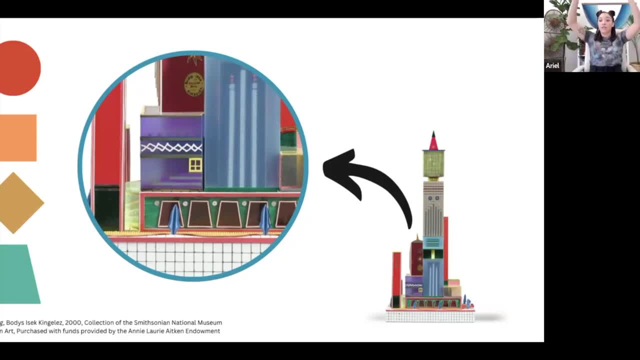 there are rectangles And I think this whole building has a lot of rectangles in it, Circles And there's a couple different circles here. There's a circle that is like- well, more like an oval, at the top of that picture And I can't really tell fully what it says, but I know it does say. 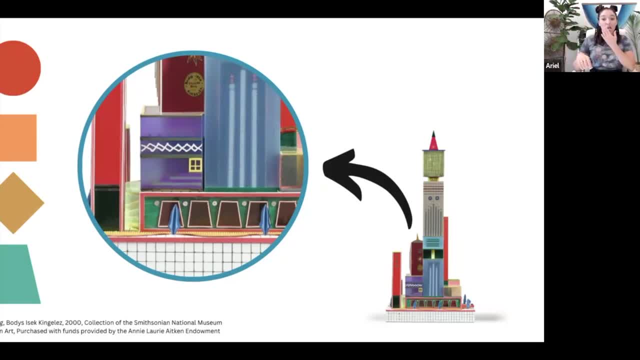 Kingalas, So it says his name on the building. And then I see those white circles that are all in a row. I wonder what those are. Someone's noticing a star? Is anyone noticing the diamonds? There's like the white diamond design. And then I see someone mentioned the trapezoid. 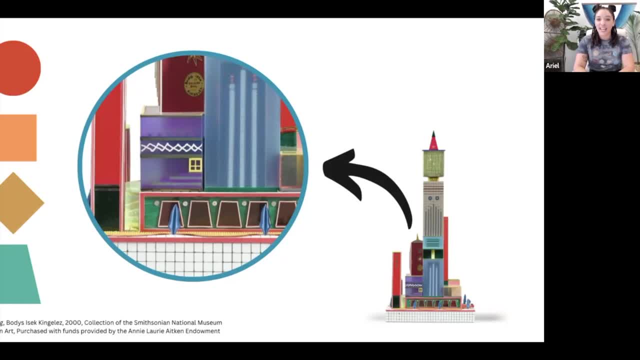 which is that green shape on our screen, And I see those big like maybe they're windows, windows or doors. But you got that right: Those are trapezoid shapes there. So we have learned a lot from our investigation so far: that Kingalas used regular materials in creative ways and that 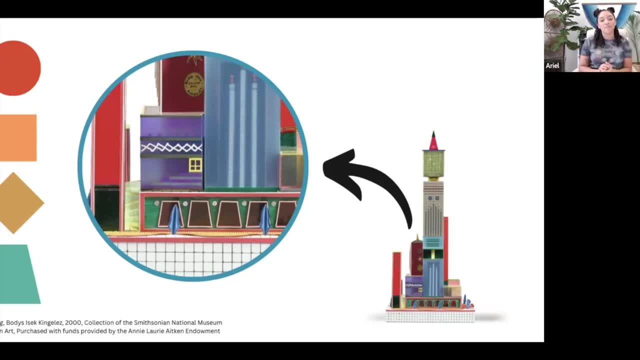 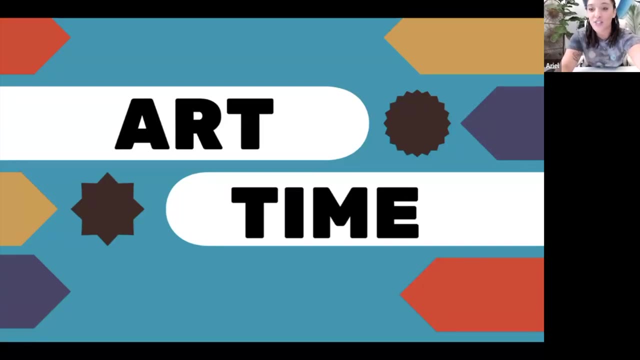 a lot of different shapes can be used in one building, And I think knowing those things are going to help us a lot as we make our own futuristic buildings. today It is officially our art time, So let's make sure we have all of the supplies we're going to need. 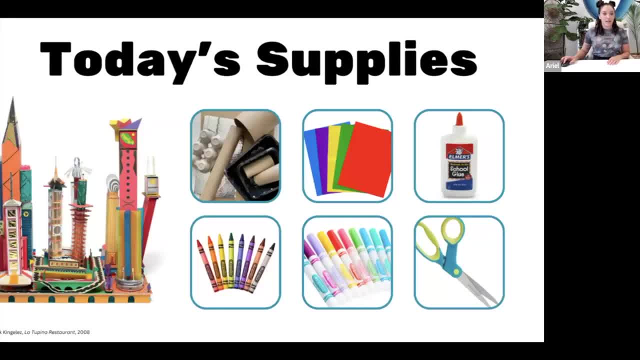 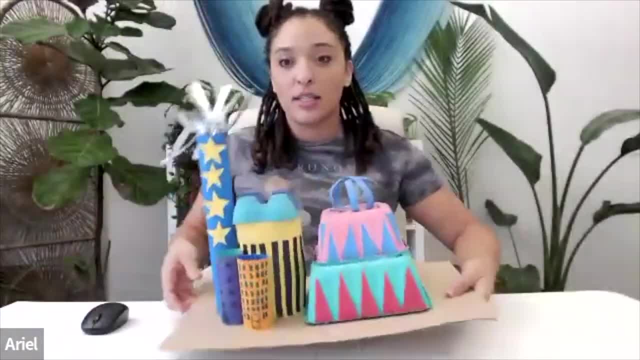 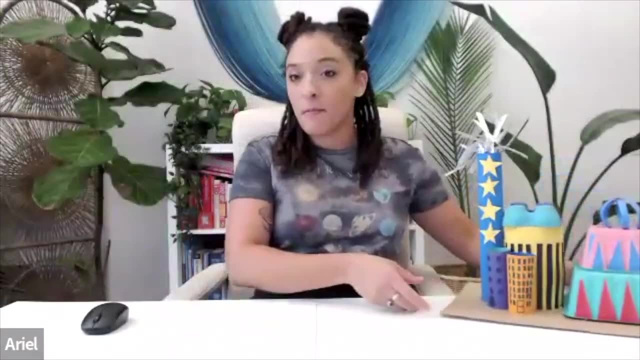 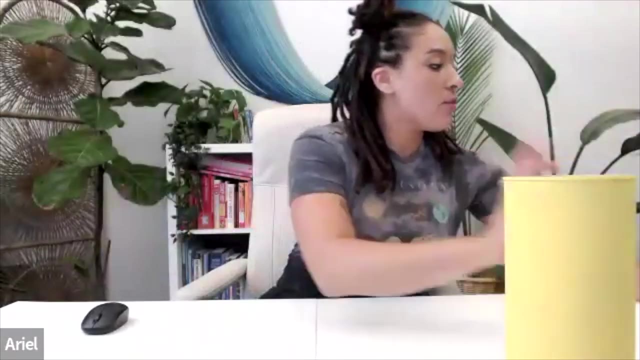 today. Okay, so today we are going to be making our own futuristic buildings, kind of like I made my own And like that one that the restaurant that Kingalas made. And in order to make our own building, you are going to need some recycled materials. Now, some friends may have brought some plain 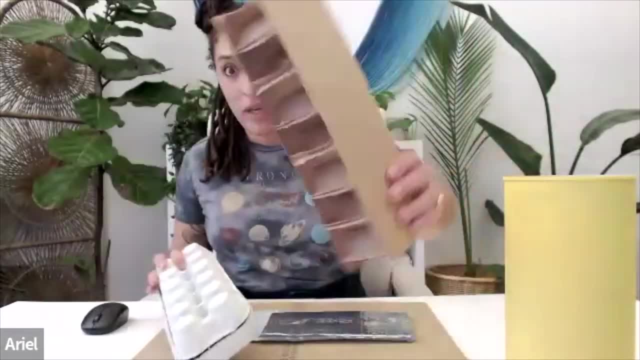 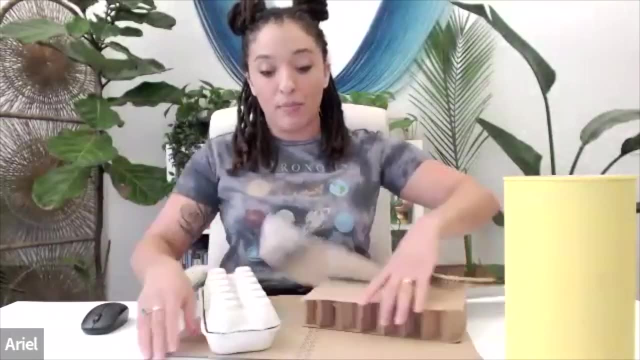 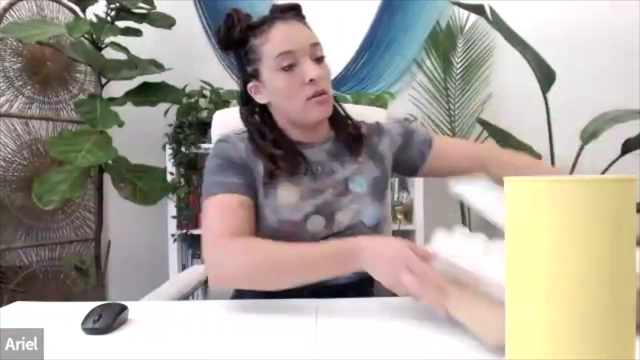 recycled materials. I have an egg carton, a big piece of cardboard, some foily, bubble wrap stuff, And I have a big piece of cardboard. Some friends may have had some time earlier to paint some pieces. If you didn't yet, that's not a problem. 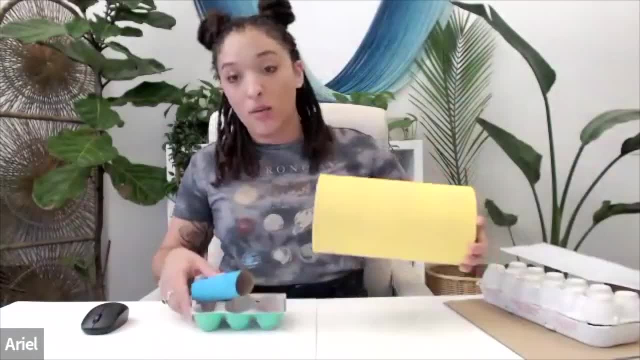 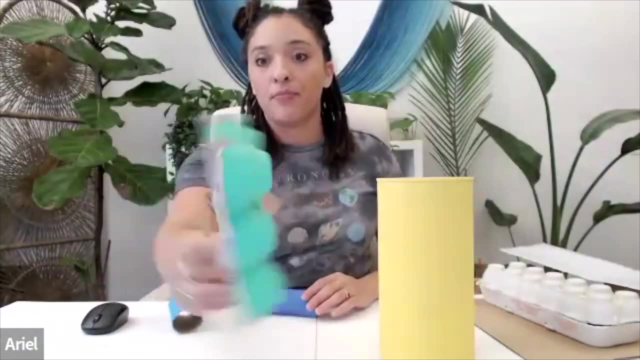 I will always bring them home. You'll always be able to do that later. But can anyone tell what this recycled material was? This was an oatmeal container that I painted, some an egg carton and some toilet paper rolls that I made. 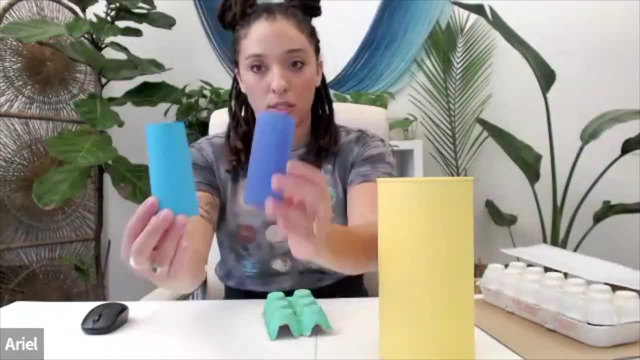 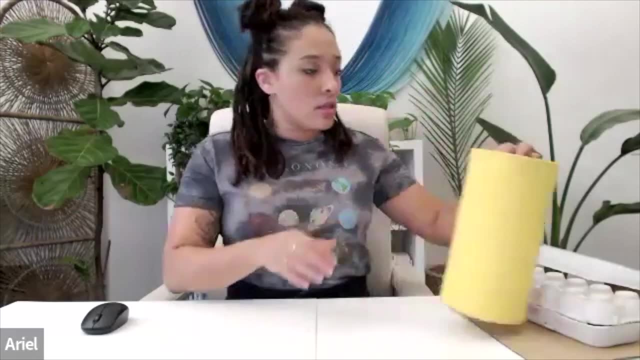 blue and purple. So do I have anything else? Nope, That's all my recycled materials. Mm-hmm, Anyway, that's all I have. That's all I have. That's all we have. That's a pretty, pretty big thing. Okay, what else do we need? We need some paper. I have some paper shapes and Ilayajima'saxou ink sacks For the base. that's really small, so that's a lot of ink. Now let's start out here to get the ink. 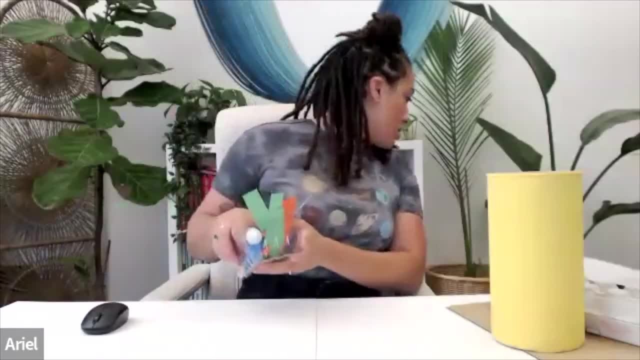 Yeah, All of those things always have to be позitive. All the LIAUANT transcend the link because of the shipping process Minus, and I had some pieces of paper somewhere. I don't know where they went, but we have some paper shapes. 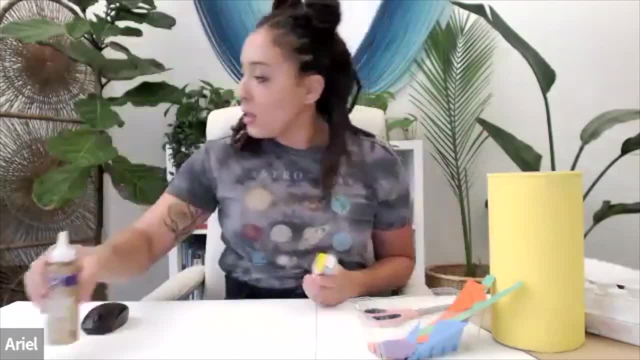 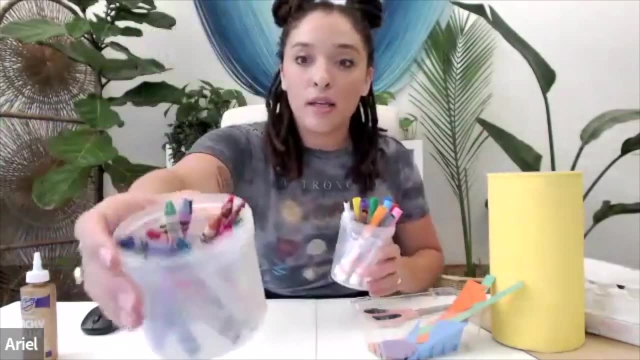 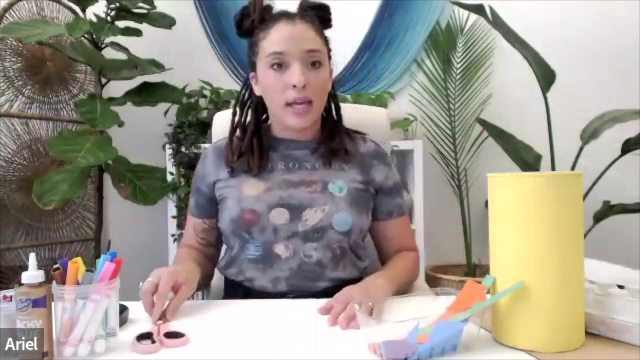 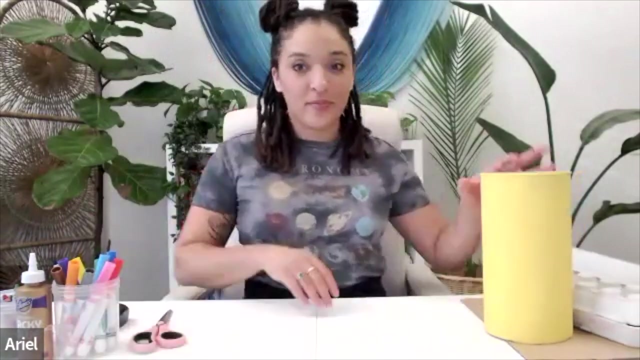 We have some glue, I have some markers here, I have some crayons- There you go- And I have some scissors And I think that is all we're gonna need to get started Now. today we are gonna make just one part, one building. 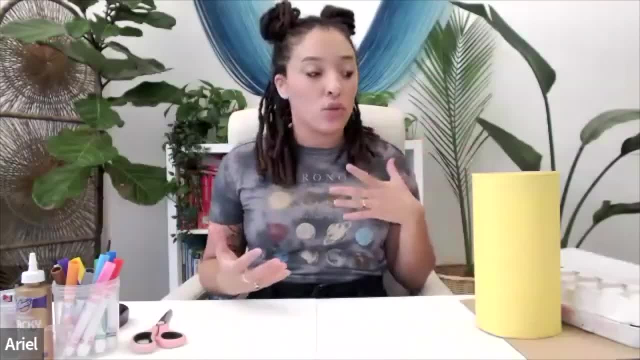 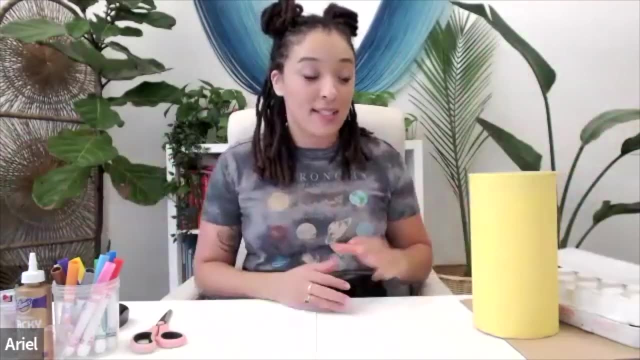 or just get started on one building, But after this you could make something even bigger, You can add more details, You could add more buildings and make a whole city. That's something that King Les did, But today we're gonna focus just on making one. 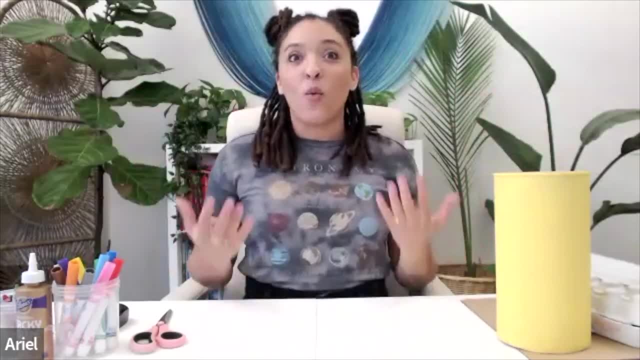 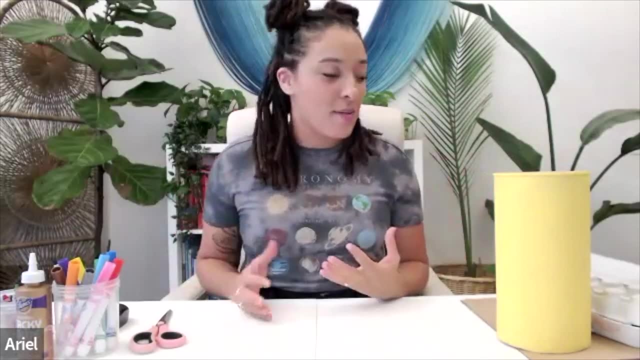 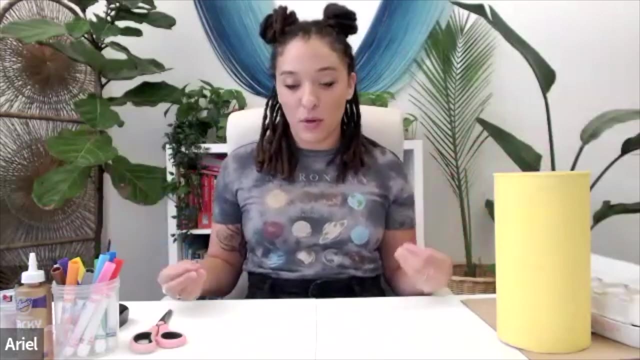 Now, the big question right now is: what are we going to make? What are you gonna make? It can be any kind of building. It could be like be looked at a hotel or a restaurant. but I want us to use our imaginations just for a moment. 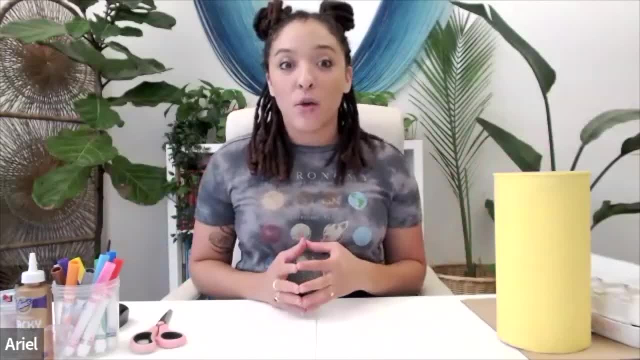 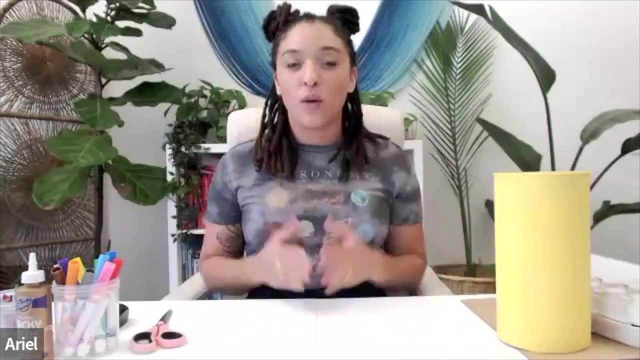 to decide what we are going to make. So, if you'd like, you can close your eyes with me. Sometimes I feel like it's easier to focus on what's inside of your brain when your eyes are closed, So you're not seeing all the other things. 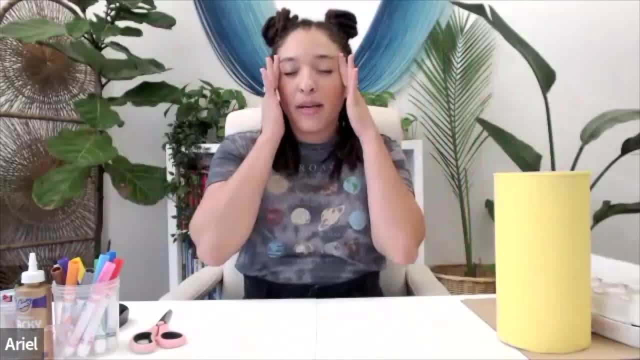 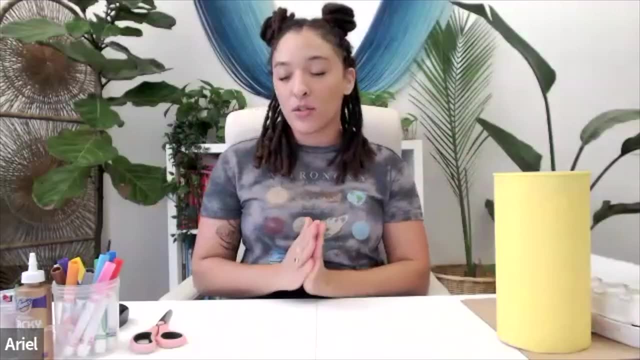 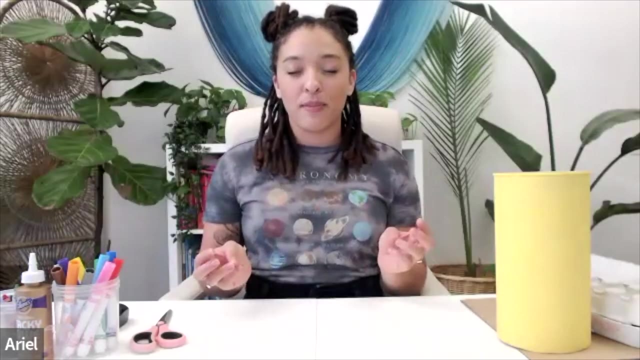 you could be thinking about And I want you to picture a building from your life. It could be your house, It could be your school, It could be a restaurant, It could be a gas station, any place- And think about. what does it look like right now? 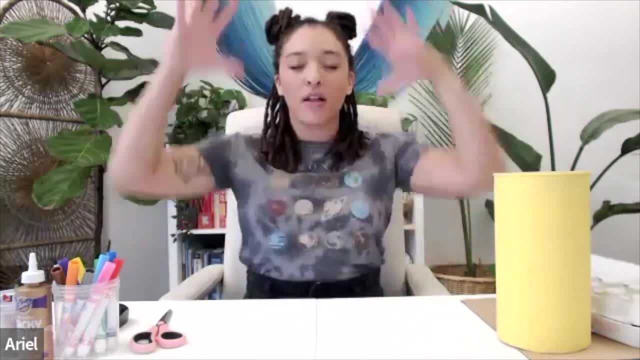 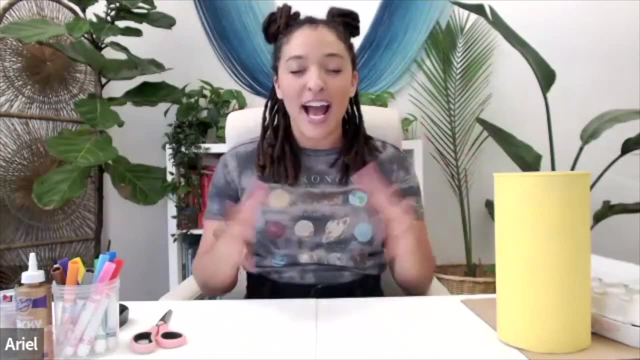 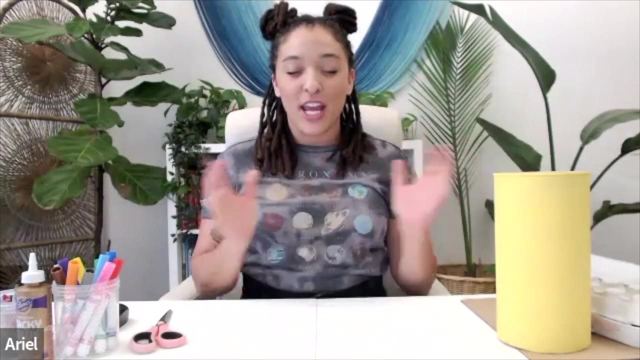 What color is it right now? Is it really tall, Is it really small? And then I want you to think about how would you change it? How would you like to change it? Is there a new color you'd like to add? Is there a different shape that you wanna make it into? 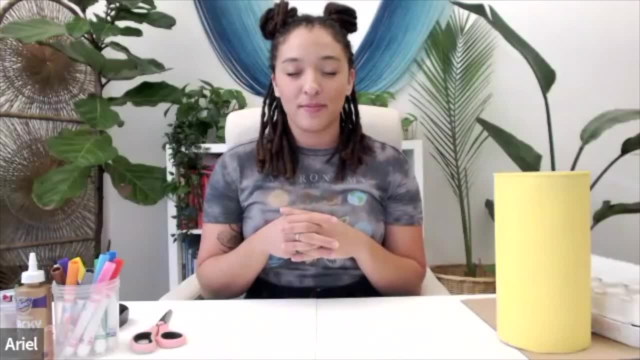 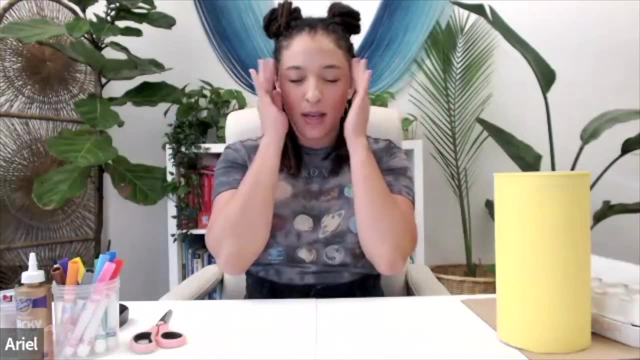 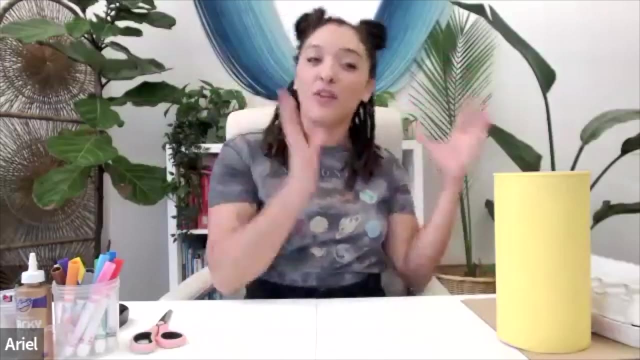 What can you do different Now? you can keep letting your brain work on that image, that picture in your mind, but for now you can open your eyes and you can take that idea, And we're gonna try and use that idea right now to make our artwork. 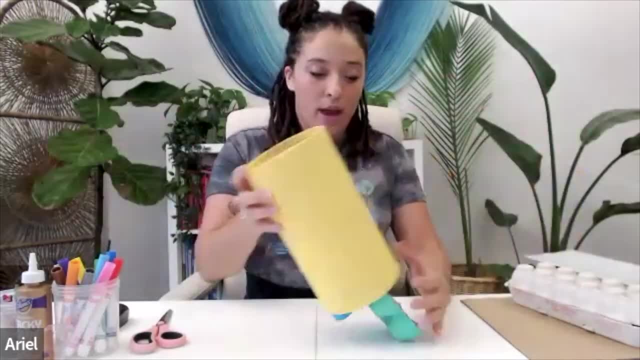 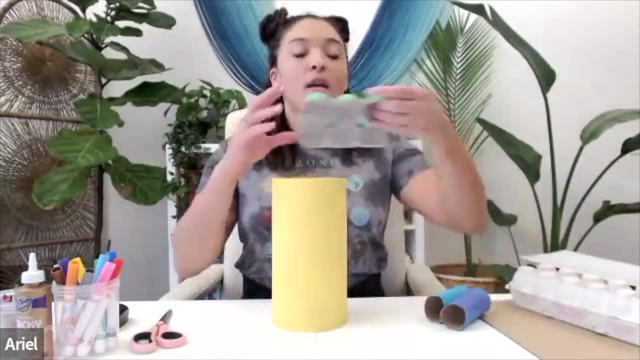 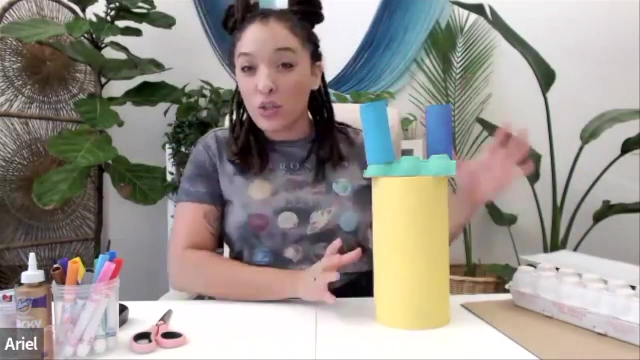 So I'm gonna start with thinking about which piece I wanna start with- that might be my main big piece- And then I'm gonna think about how later I'm gonna add on some things onto my building. So I'm not gonna glue it all together. 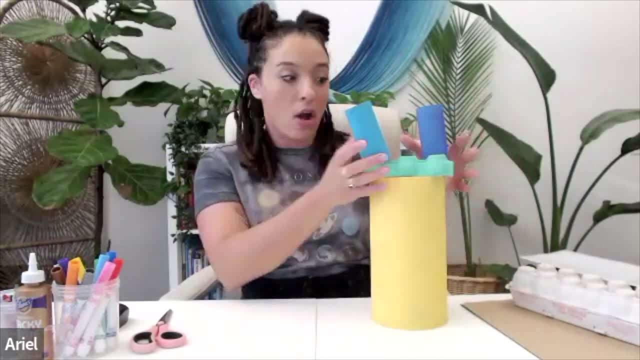 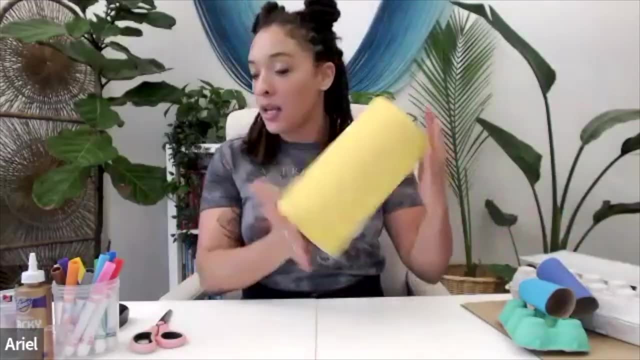 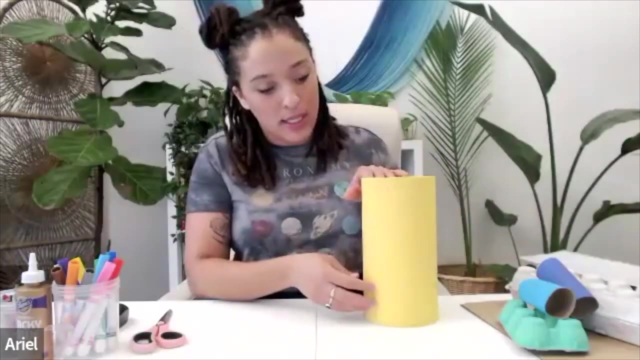 I wanna decorate my big piece first and then add on things. So once you pick your big piece- I picked my oatmeal container- I'm gonna think about what do I wanna add on top of it? What kinds of things do we know buildings need? 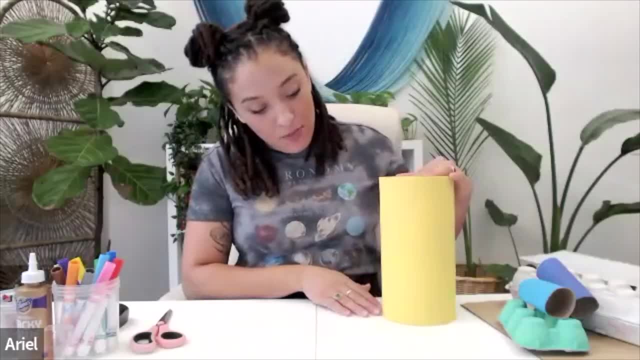 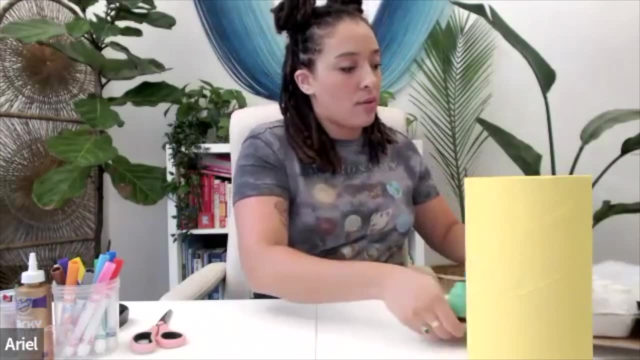 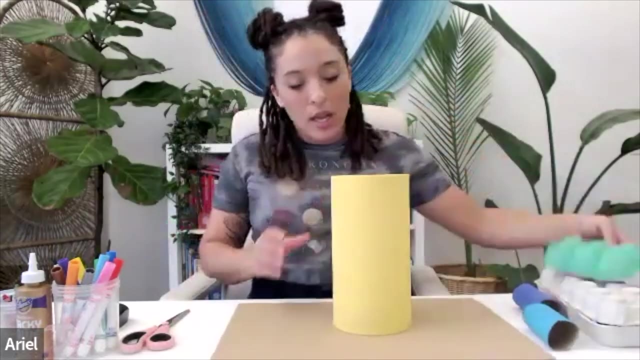 Like windows and doors, It needs paths to get to it right? Let me make sure I'm gonna put this on top of this big piece of cardboard. so I work on this. There we go, Okay. Okay, I think what I'm gonna do first is add some windows. 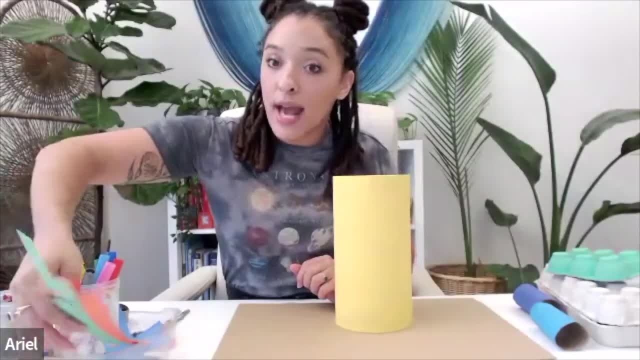 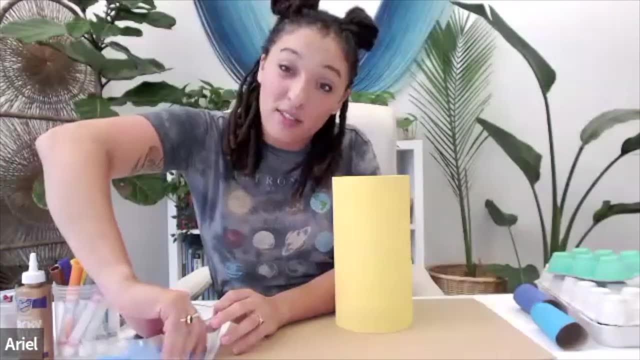 Now you may need to cut these shapes if you don't have any yet, or you might already have some, but there's some square. I think I would like my windows to be squares, and maybe some diamonds, So I did cut some little squares. 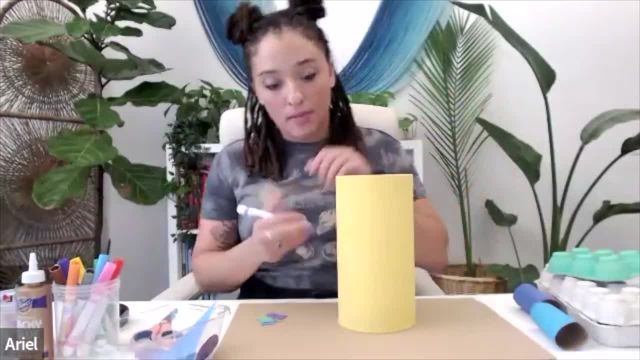 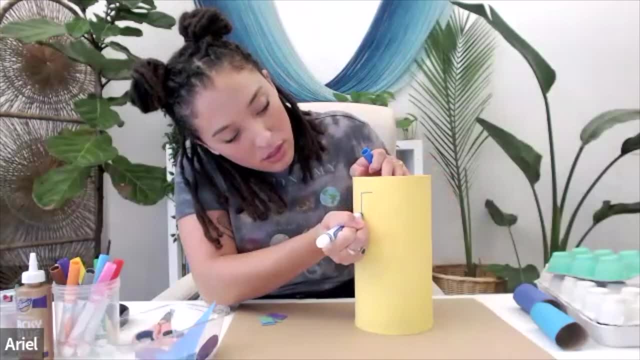 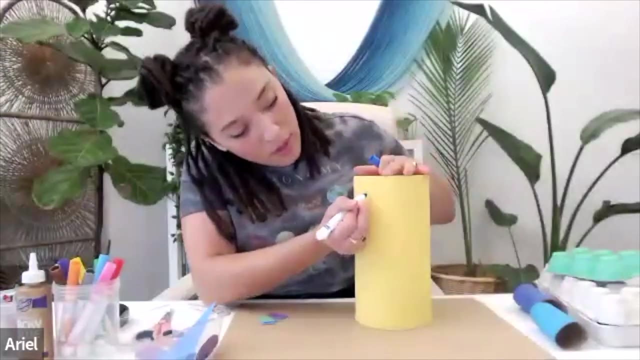 but I could also draw on some. So I'm actually gonna draw and then maybe glue on some too. So let's see, I'm just gonna. you see that one. There we go. Now these are some big windows. Oh wait, I didn't even tell you what I'm gonna be making. 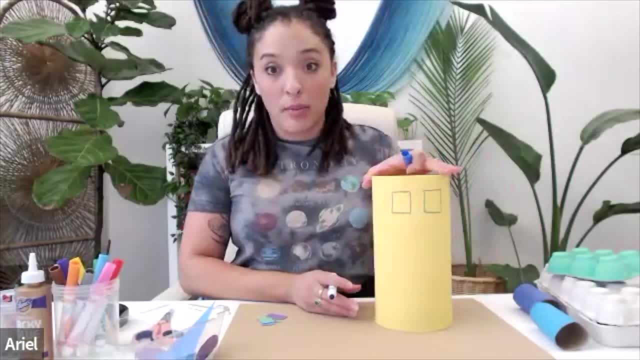 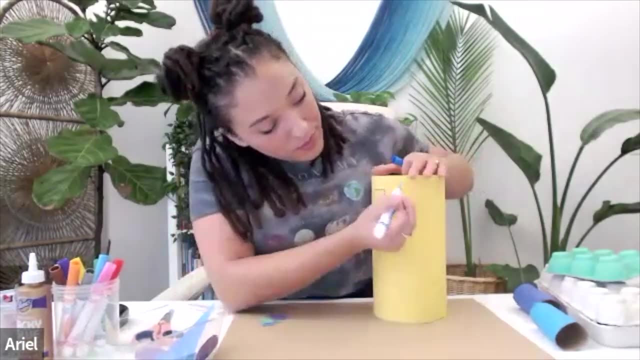 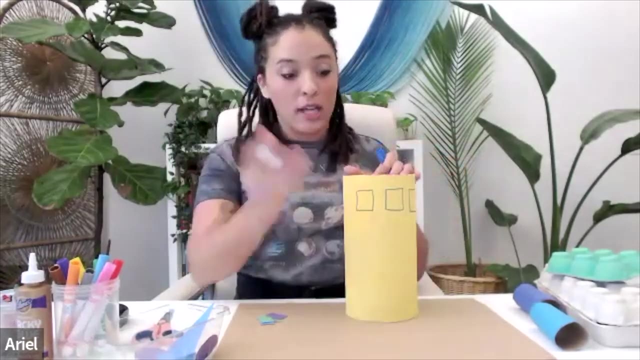 My building is actually gonna be a hair shop. It's gonna be like where I can go get my locks done, okay, So I would love, when I'm waiting and getting my hair done, if I had some big windows I could look out of. 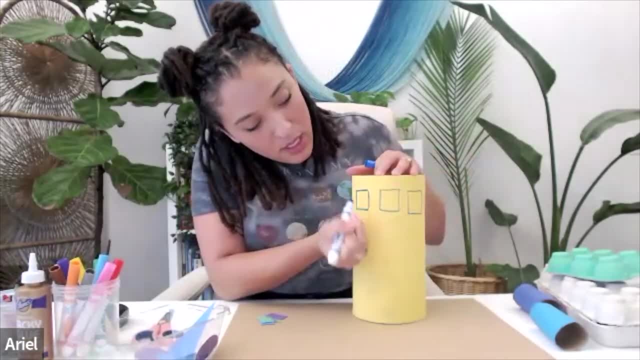 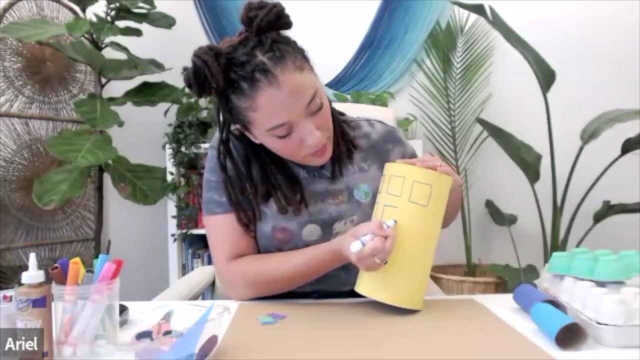 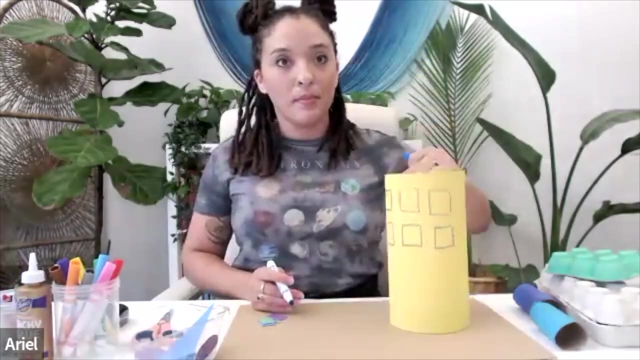 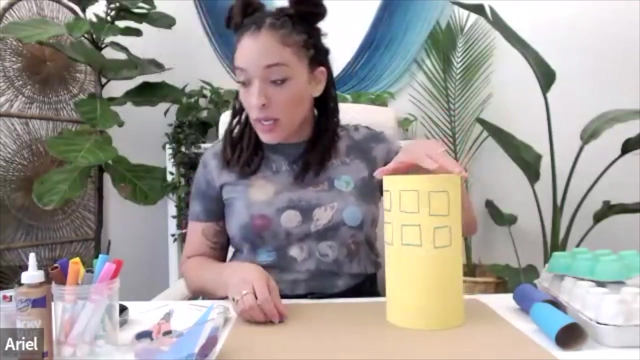 and look at all the birds flying by and the sun and the clouds. while I'm waiting, while I'm getting my hair done and getting my hair washed, What kinds of buildings are you all making out there? You gotta let me know what our 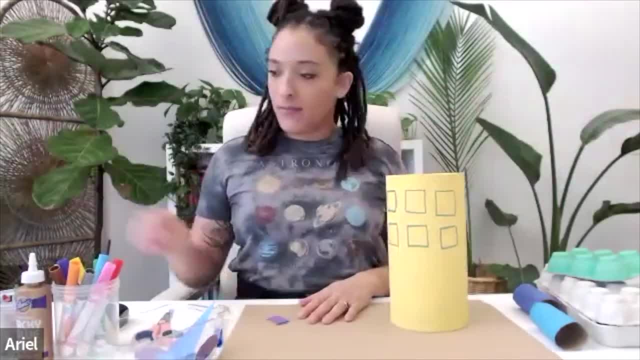 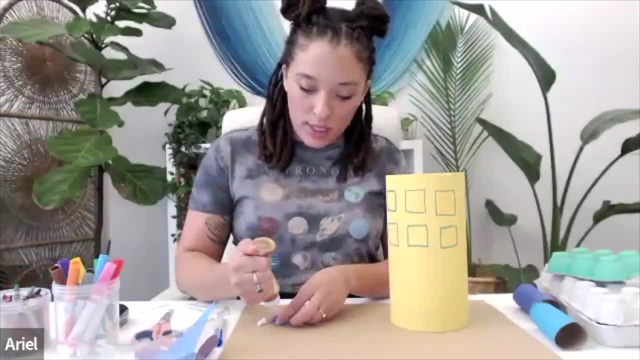 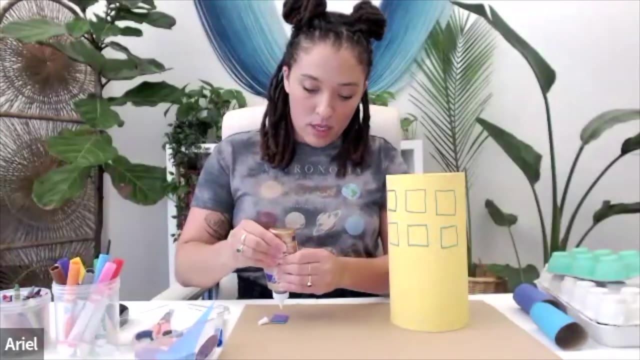 I guess virtual city we're building together is Now. I am using wet glue because that usually helps stick on a little better than blue sticks, But, as you can see, it does take a little bit of extra squeezing If you're using wet glue. 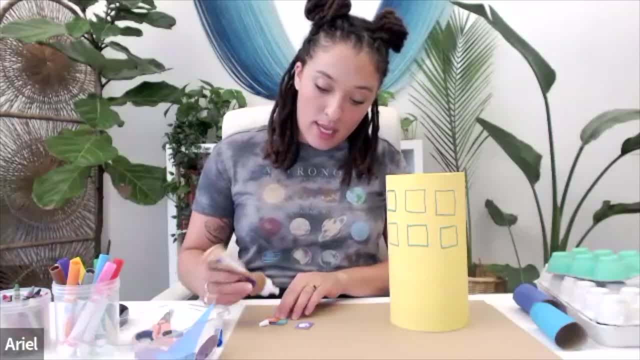 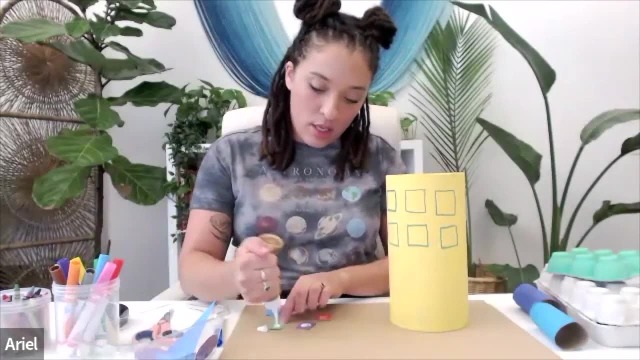 especially for adding on the paper. I like to say I'm adding some glue in my brain, dot dot, not a lot, Don't need that much to help it stick actually, So you don't wanna do too much glue. Does anyone know that book? 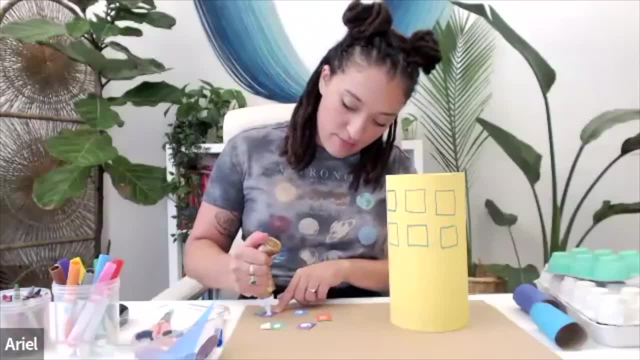 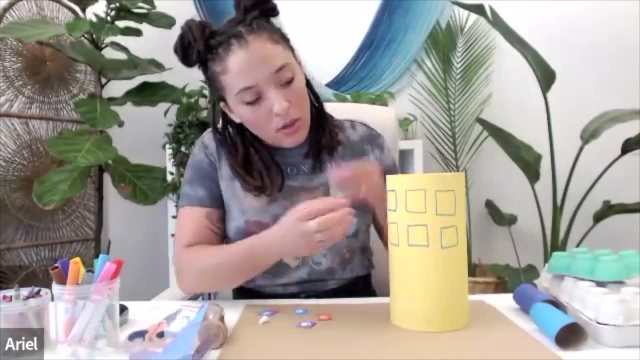 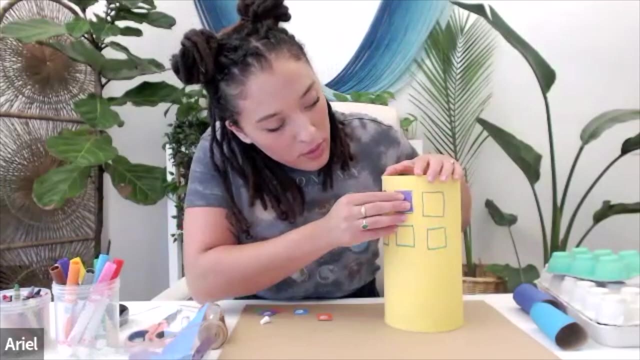 too much glue. That's one of my favorite ones When you're using glue and it gets a little out of control. Okay, So now I'm adding some shapes to all of my windows and I'm adding a little bit of color to them. 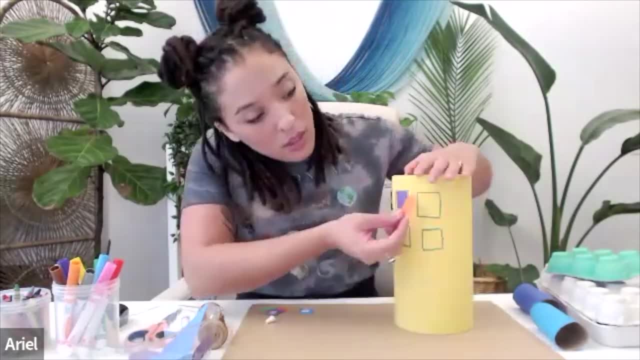 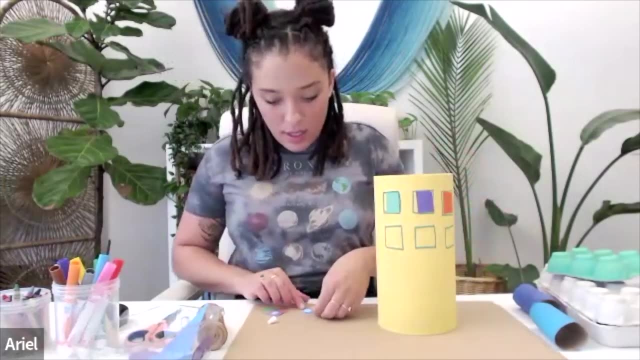 I used a green window, I used a. I'm using an orange, making an orange window. Oh, that would be cool If the glass was different colors. So when I look outside, it's not just regular color, It's just it might have a little tint of blue. 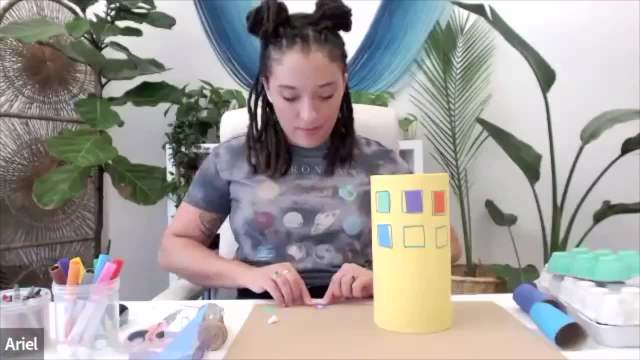 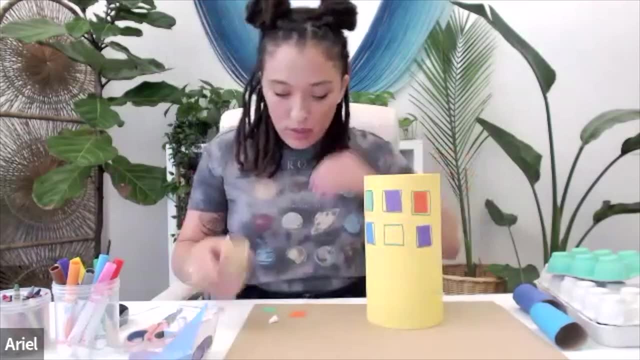 Someone out there is making a condo building. I wonder how many condos is in the one bill. Oh wait, I got there. There we go In one building, Okay, Okay, And you have to. and then you think about what kinds of things do people need? 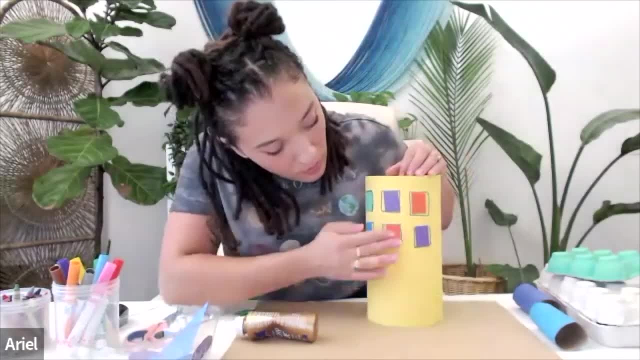 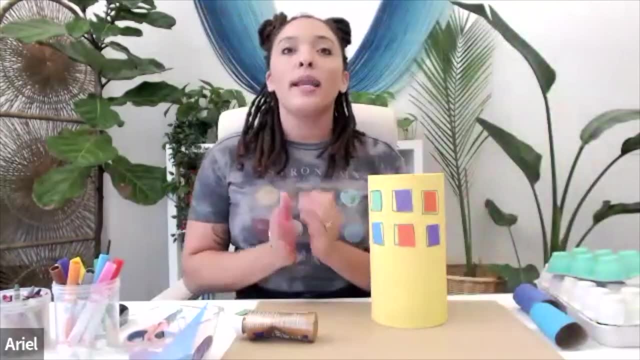 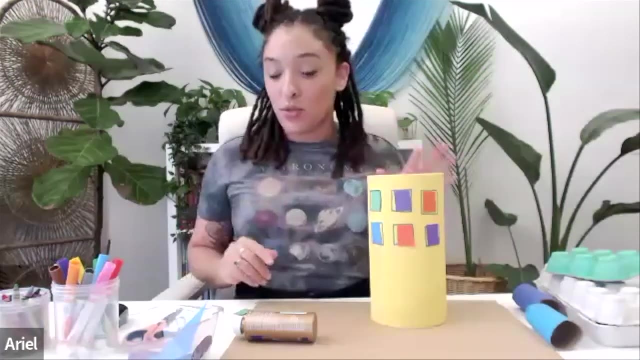 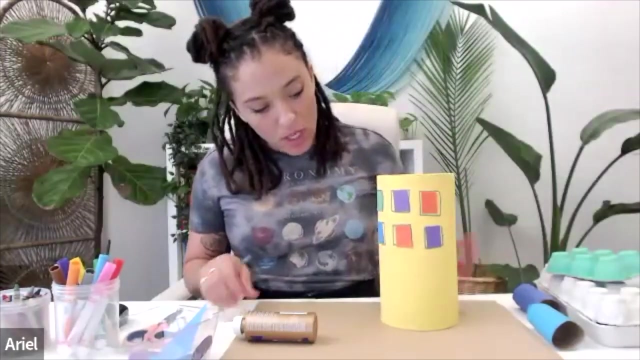 at a condo building. Okay, I have some windows on my building. What else do I need? Hmm, One thing that people do need is a way to get inside of my building, So I'm gonna create some doors, And since this is a pretty tall building, 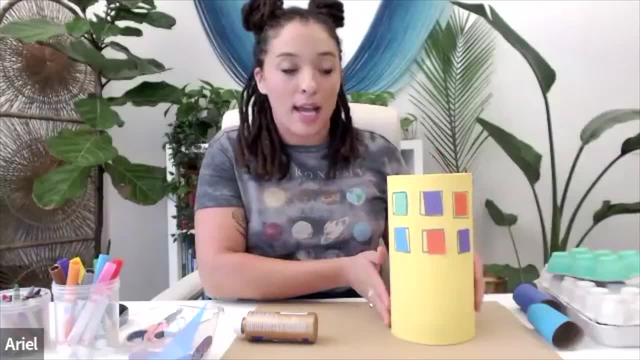 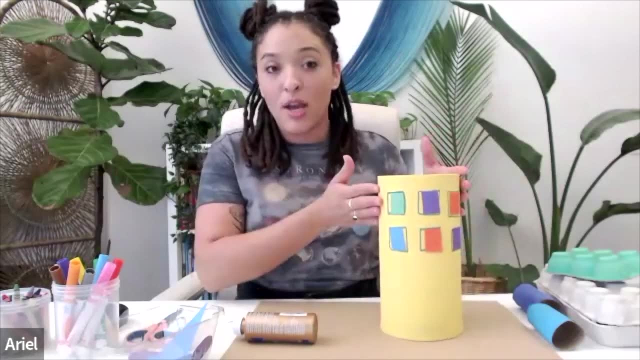 there's probably gonna need to be some stairs inside of here, So maybe I could make some stairs If I use my imagination. of course there's gonna be some stairs in there, but my imagination also wants to say there could be like a slide. 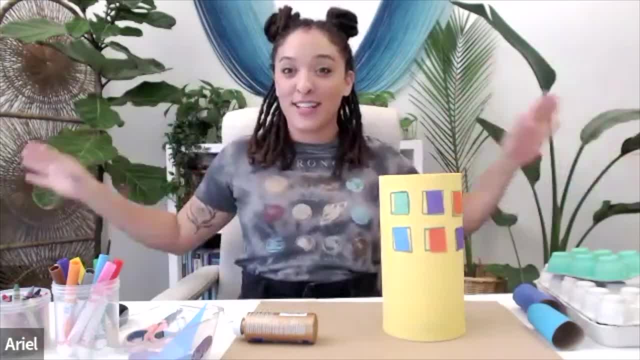 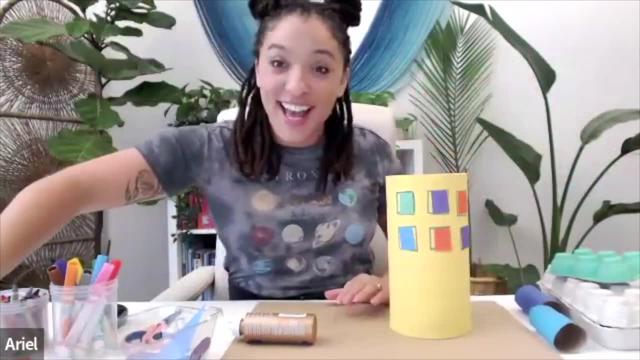 How fun would that be That when I'm done getting my hair done, I could just go down the slide and out and go home. That'd be kind of fun. Okay, Let's try and make that, We'll see. We'll see how it turns out. 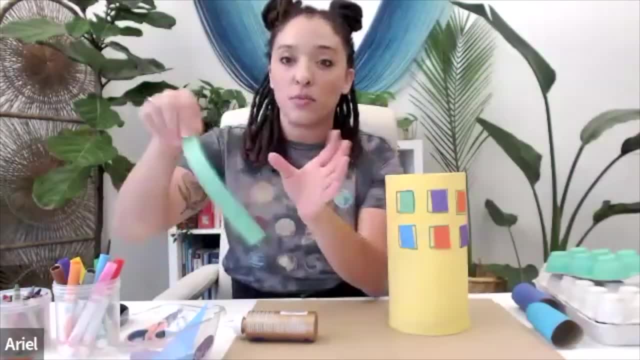 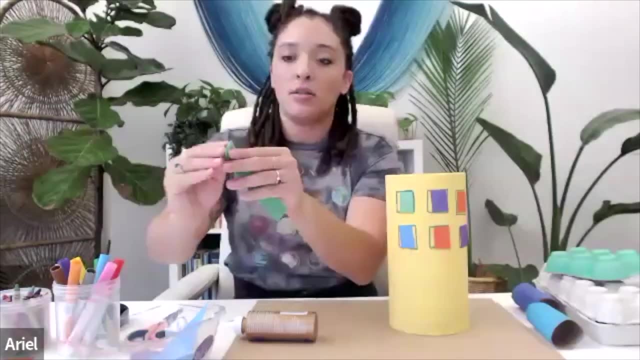 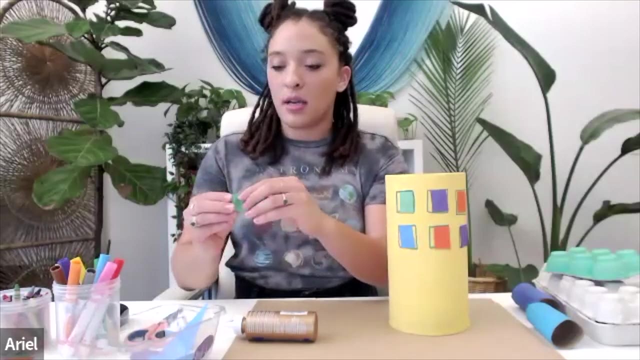 Okay, So for some stairs, my idea is I'm gonna take a strip of paper and I'm gonna bend it like this. Let's see if you can see that little zigzag kind of shape And that kind of looks like stairs to me. 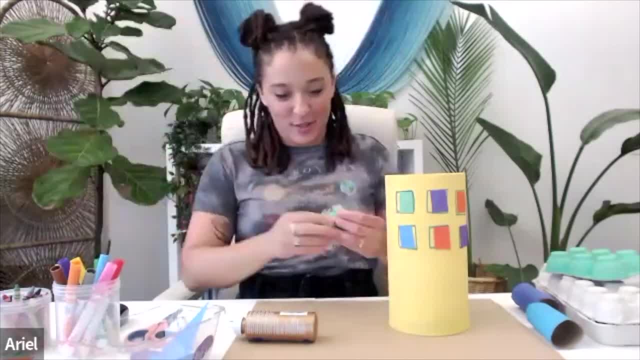 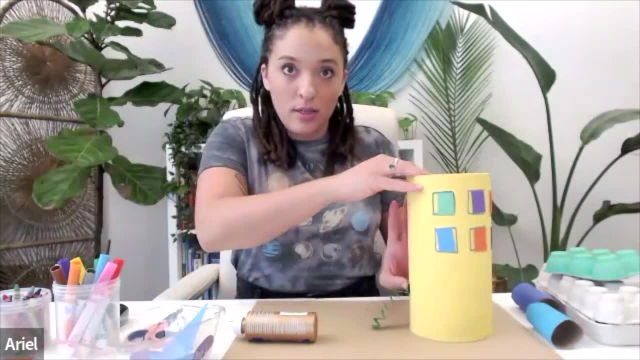 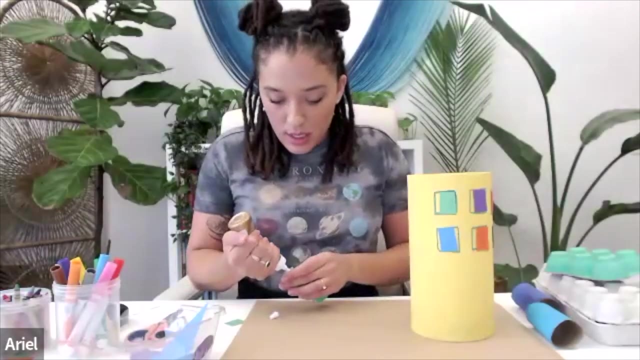 Like that. Yeah, I think that's gonna work well, Okay, And I just have to, I guess, glue it to the side here. Can you see that? well, Let's see. Someone just told me a new kind of building they're making. 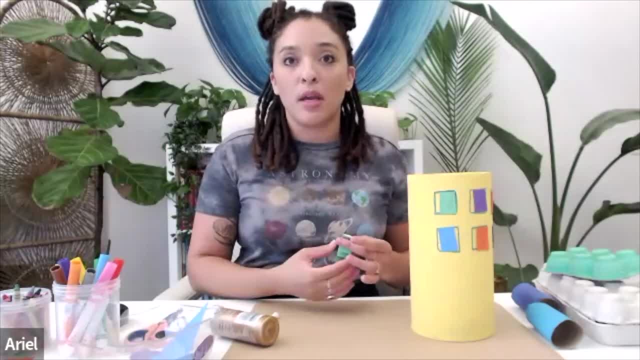 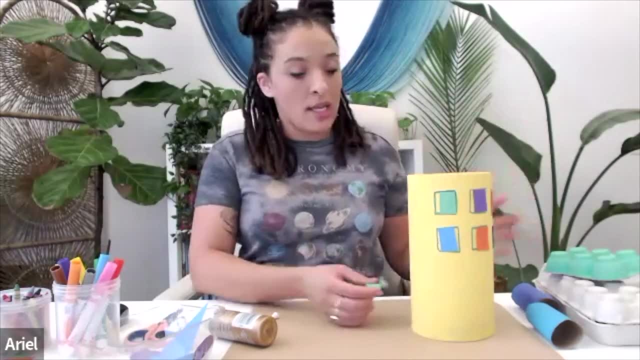 It is a building with a restaurant and people sleep there and they have school supplies there. I mean, that's everything that I need. I need to be able to eat, I need to be able to sleep, Let's have some supplies so I could do some work and do some art. 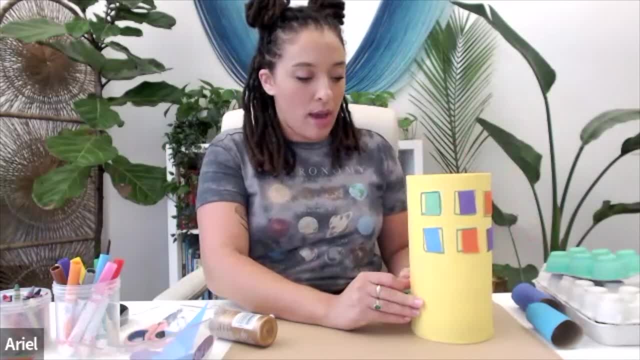 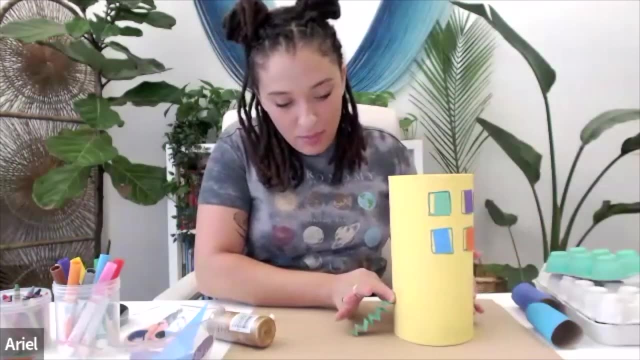 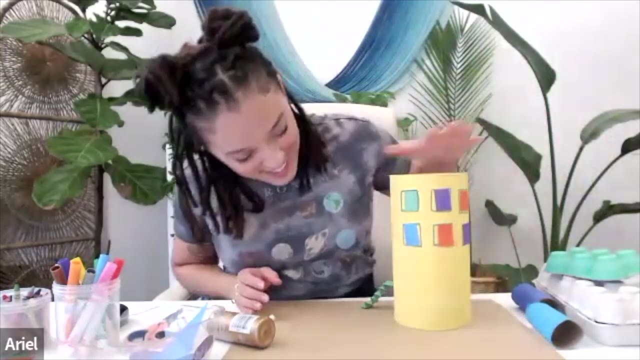 So I like that idea. Very strong imagination there. Okay, Oh my gosh, This is turning out really great. I'm really happy Oopsies I'm really happy with. Look at that staircase. Whoa, that's really cool. 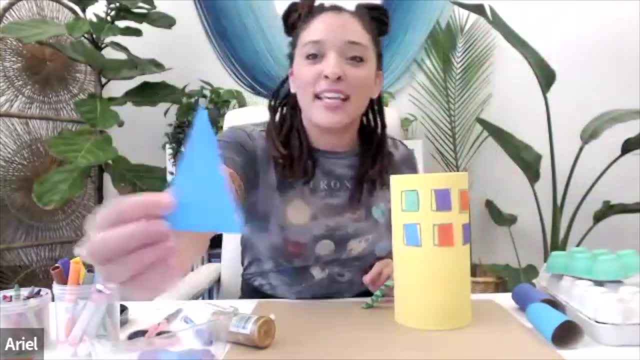 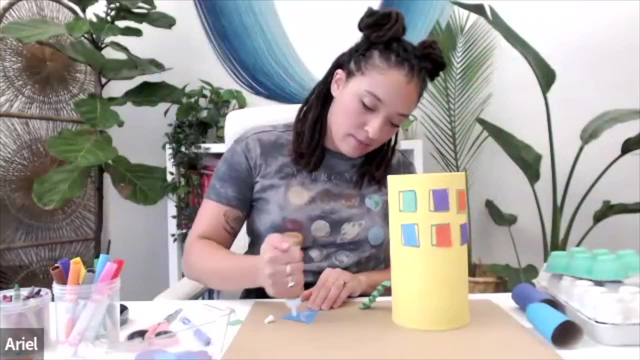 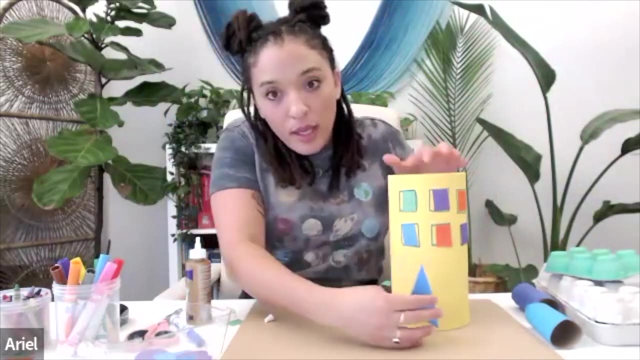 Okay. Well, now I need some doors. I think that to be a little bit creative, I'm gonna use a triangle as my door instead of a normal rectangle kind of door, And let's see- Oh, let me try and put it right in the middle. 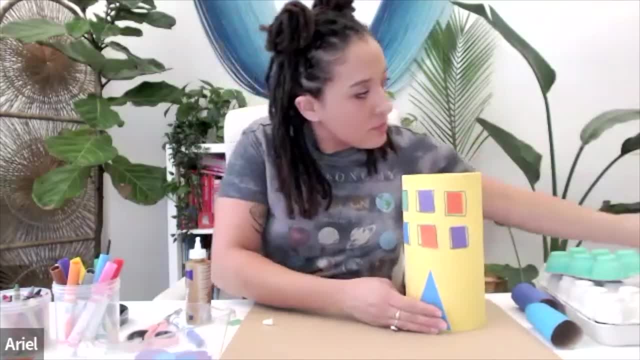 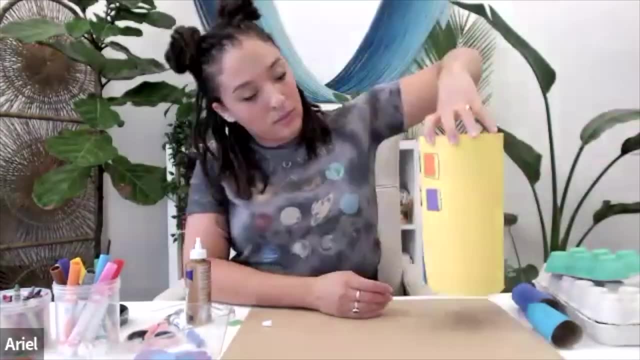 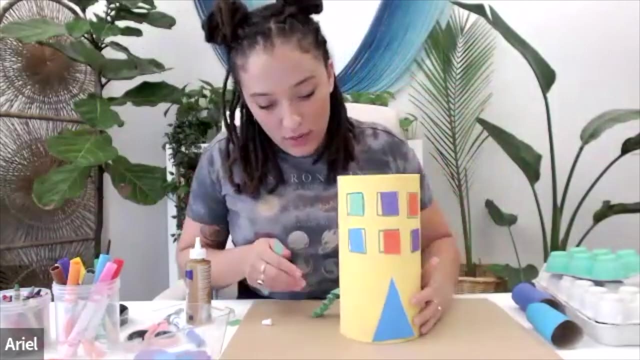 Put it right in the middle. There we go. Okay, Oh, I forgot. I said I wanted to do a slide, So maybe, Oh, you know what friends, What? if? Okay, The people can walk up the stairs on this side of my building. 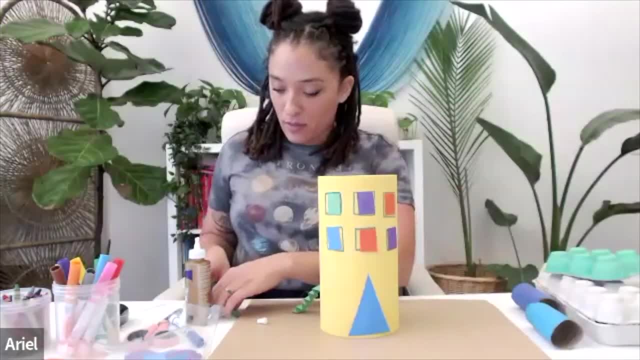 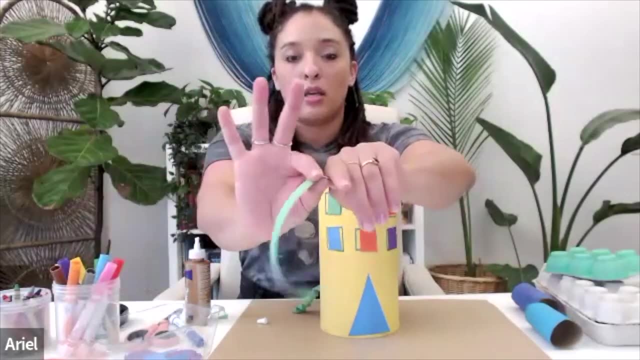 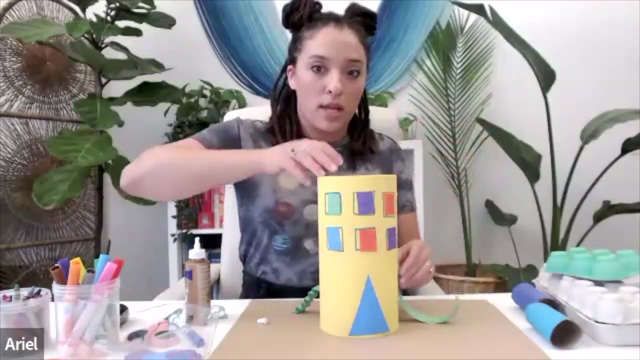 And then on this side of the building they can go down a slide. Let me try that. So one way that you can sometimes curl a piece of paper is, if you kind of like, pull it and turn it And then if I glue that to the side here. 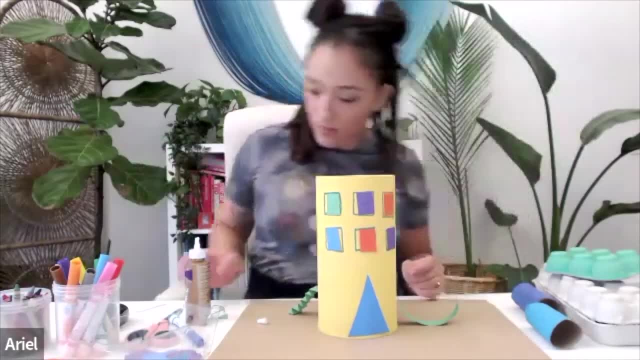 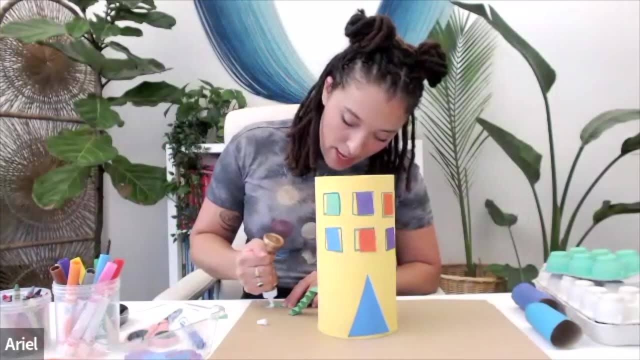 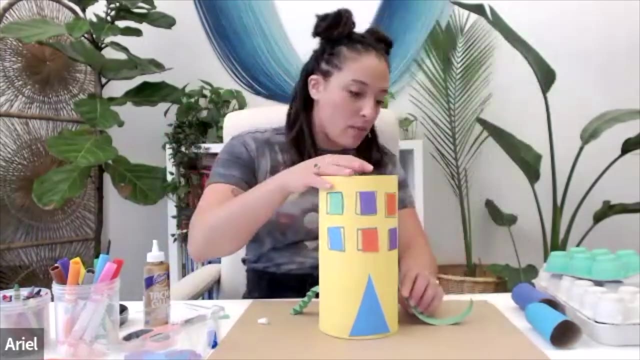 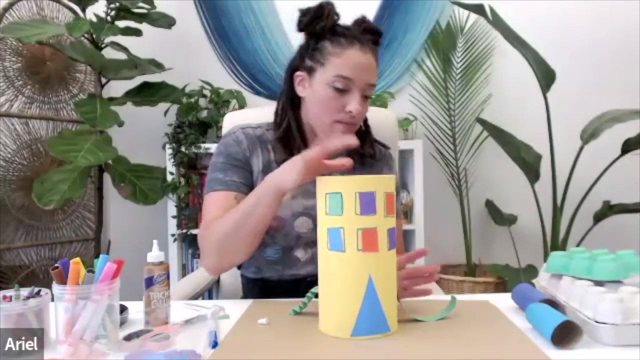 that looks like a pretty fun slide. Yeah, Now, what colors are you all using? I'm imagining that, with all of the inspiration we got from Kingalas, that people might be making some pretty colorful buildings on your side of the screen. 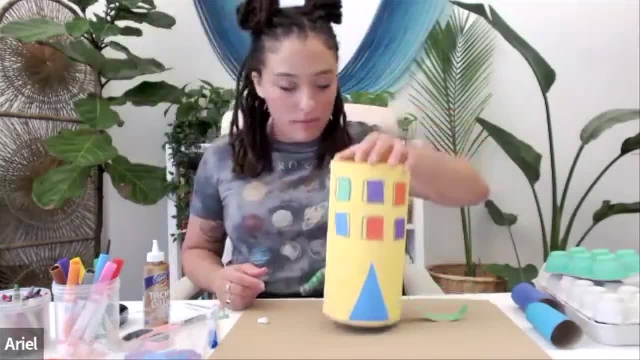 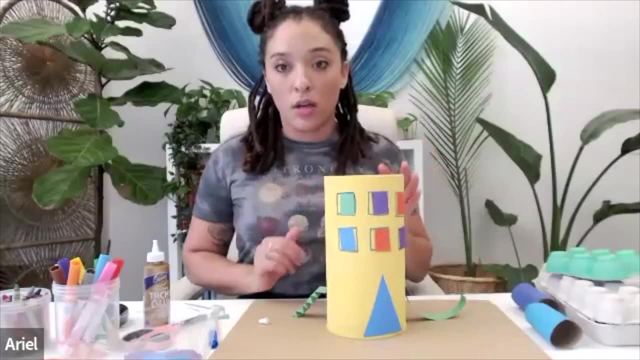 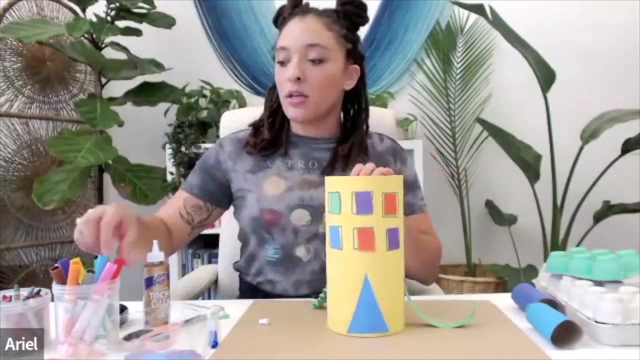 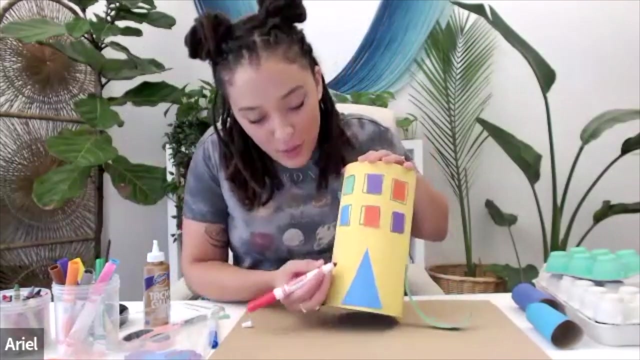 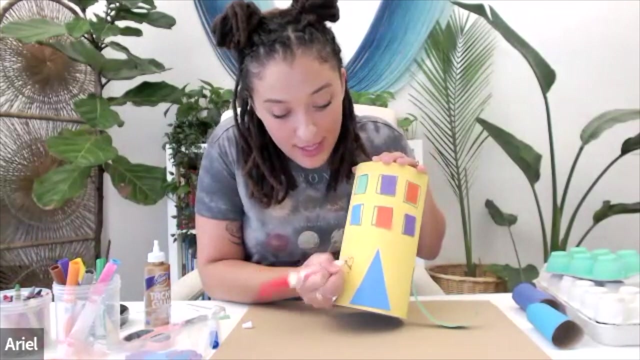 I've used like five different colors so far. Okay, Any other things that we should add to our building, Any other details? I guess I could add some decorations. So someone is building a rock tower of pizza. That sounds amazing. That sounds. 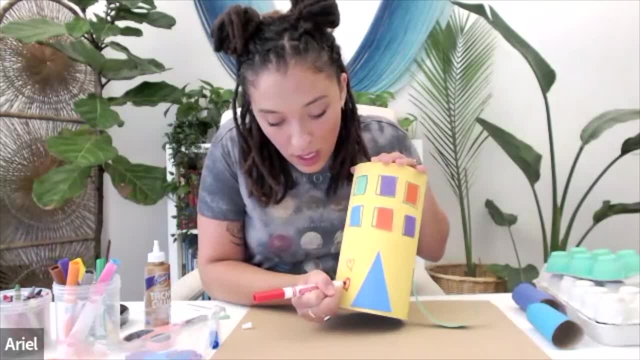 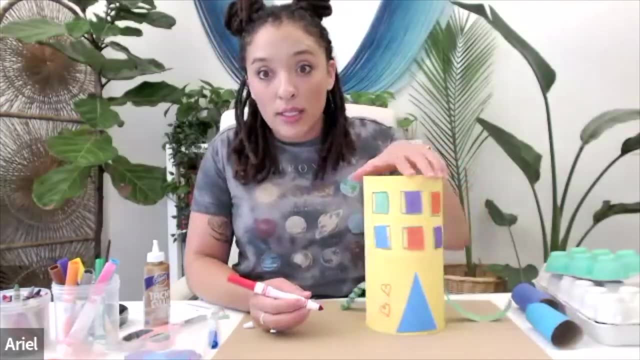 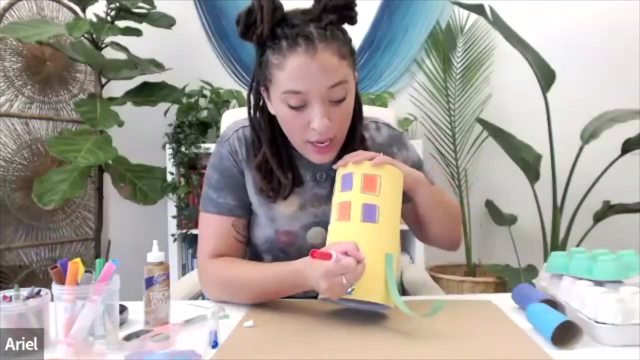 Pretty good. I'm wondering in the tower, how many floors are in the tower And then on each floor, is it all just pizza, Just like different kinds of pizza. Can you do different things on different floors of the tower? Different kinds of pizza available on different towers? 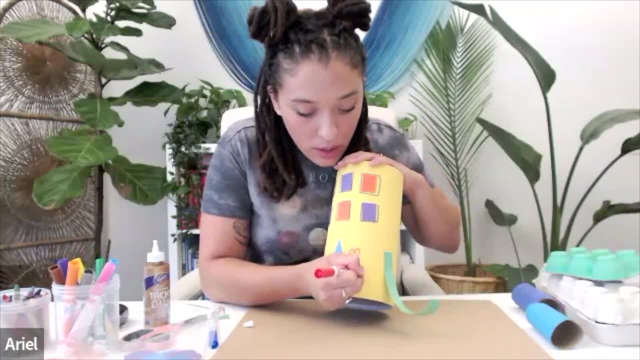 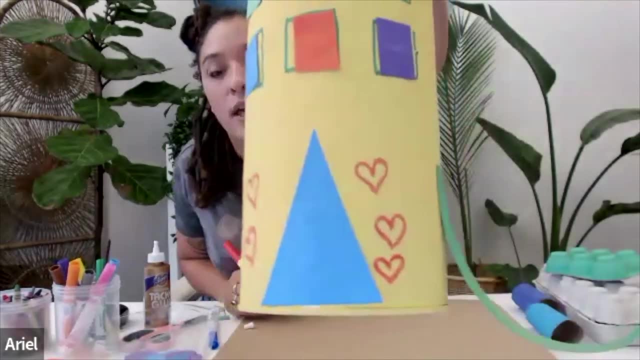 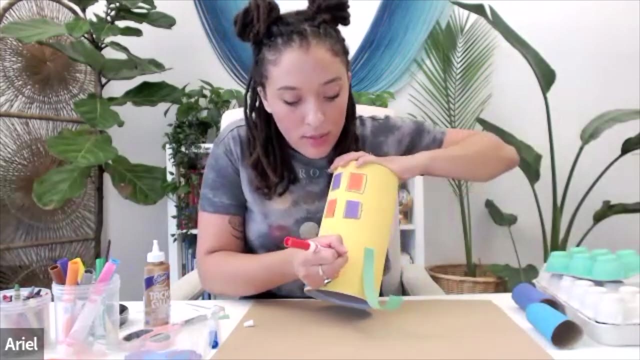 I mean, your imagination can just keep going and going. Okay, I decided to add hearts because I love my hair And I want, And other people who might come to get their hair done, you want them to love their hair too. So maybe, if they have hearts on their way walking in, 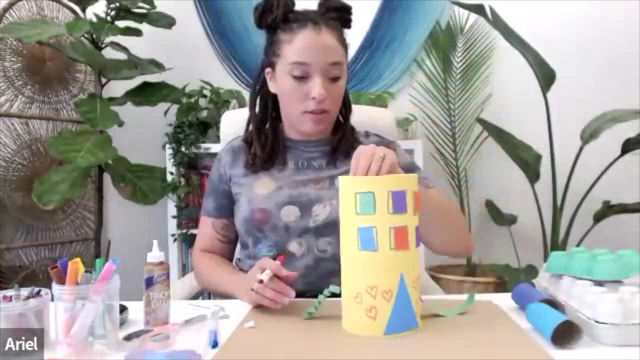 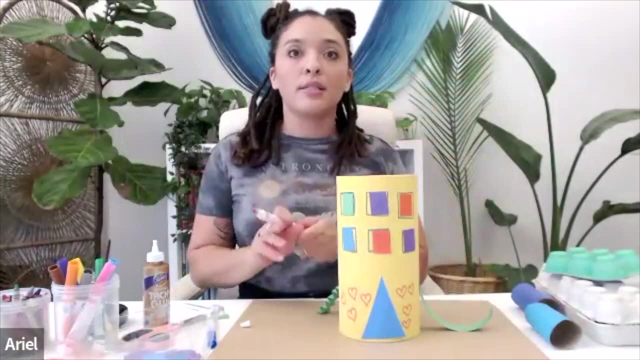 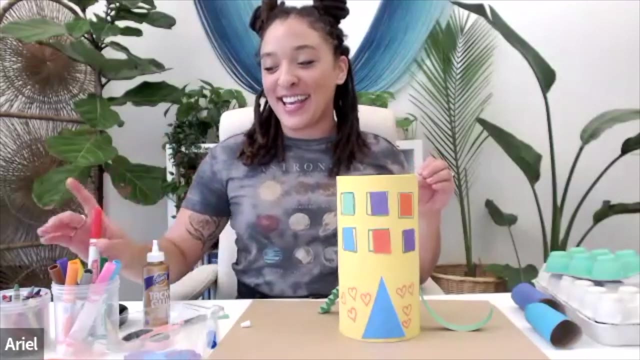 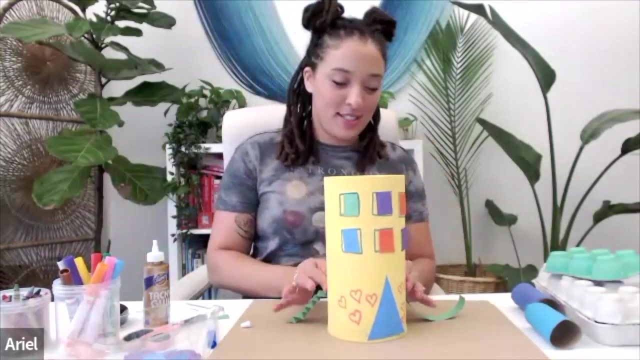 they're going to feel really, really happy and proud of how their hair is. Okay, Let's see, Oh my goodness, Someone is making a zoo. I think that is an amazing idea. How fun, Oh my goodness, I love the zoo. 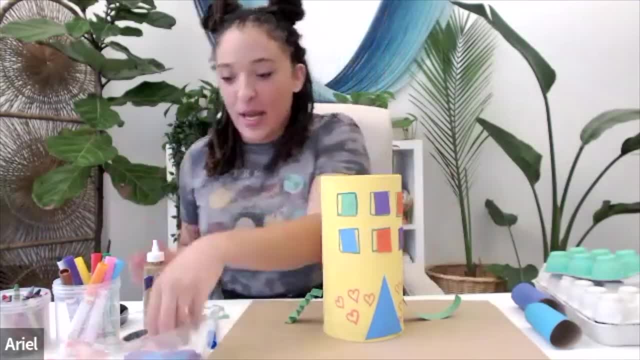 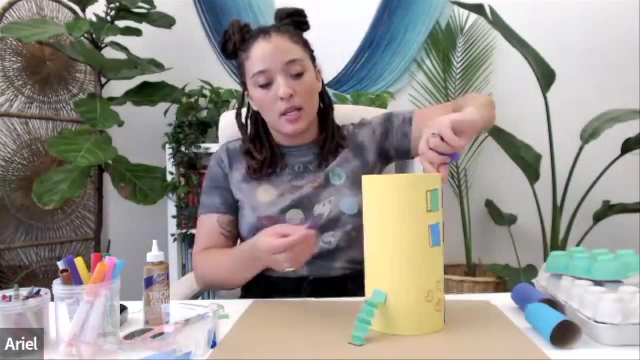 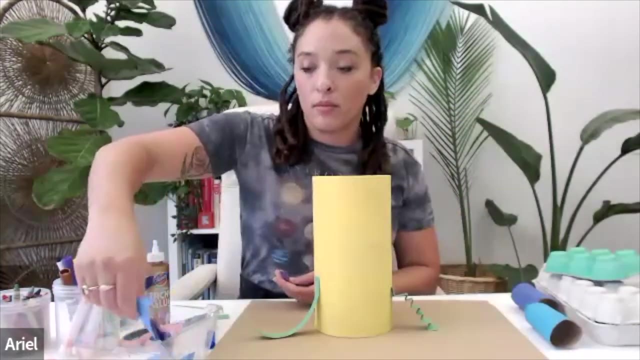 I'm so curious what you are imagining. over there it looking like Now. of course, on the other side of my building it doesn't have anything yet, So I could add. I might add some circle windows on the back, So I might add that really quick. 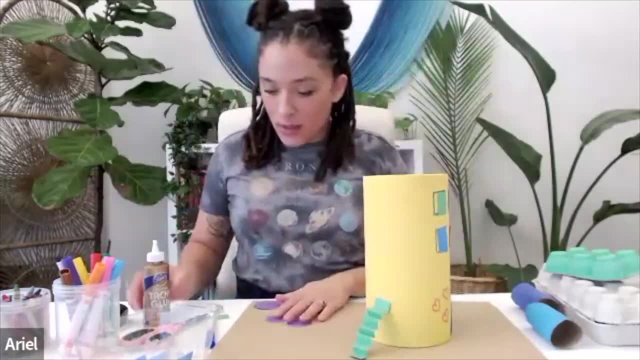 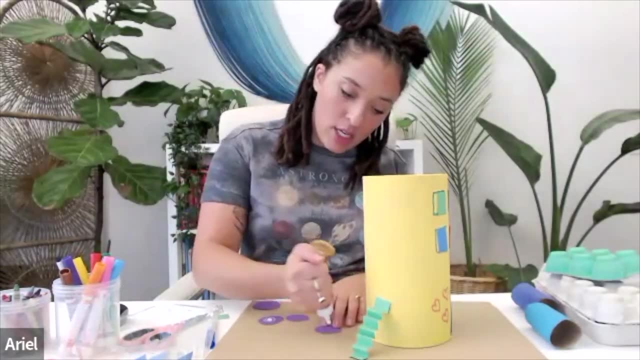 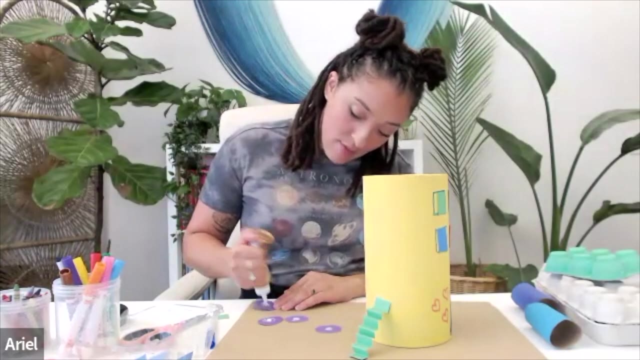 Okay, Now, the thing, friends, that I really like about making art is- and ultimately, using our imaginations- is that it can really be anything that you want. You just have to be brave enough to think of it, to think different. 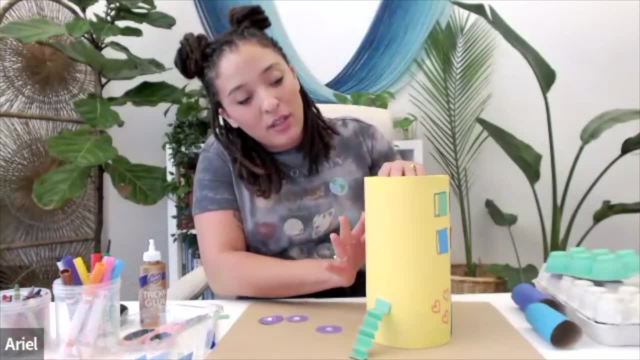 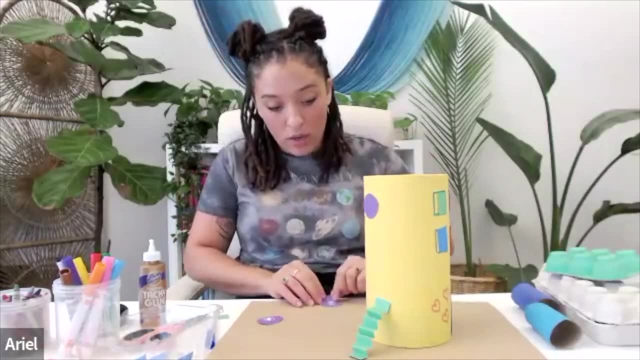 Sometimes the future can kind of feel make you feel a little bit nervous sometimes, because you don't know what is going to happen. You don't know where you're going to go or what you're going to do, But our imaginations kind of give us some power over that. 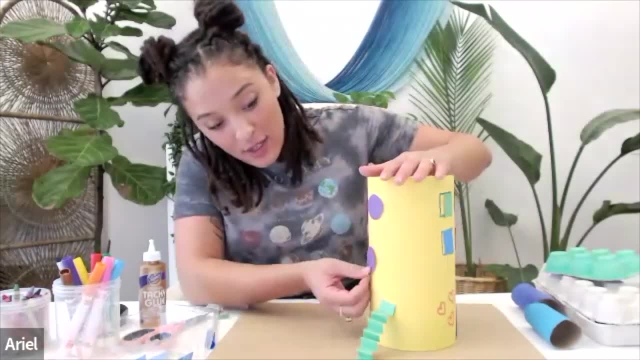 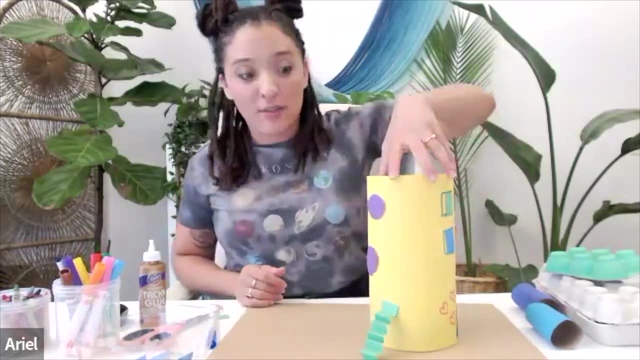 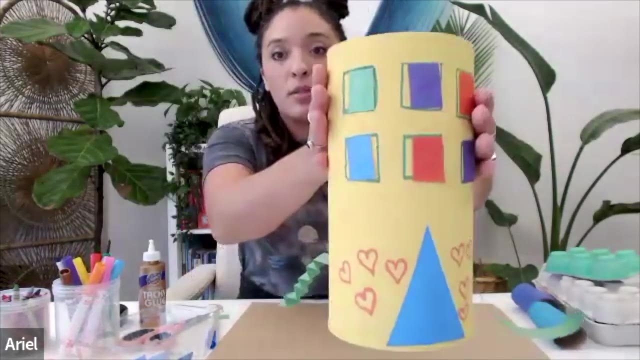 Our imaginations help us to decide what the future can be, And it can be a lot of things, And you get to have a little. you get to have some say in what it's going to be. All right, That's what my building is looking like so far. 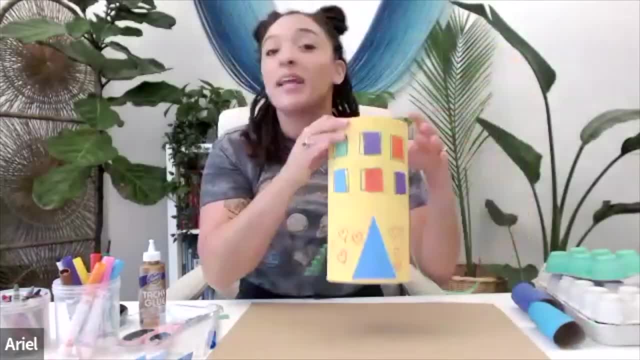 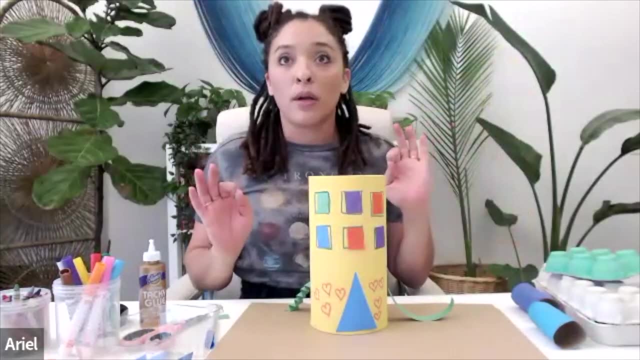 It has a lot going on, but that's a very Kinggla style of doing buildings, so I'm feeling really good about it. Now, before we're we're coming to the end of our program, so I want to make sure I do some of our last steps. 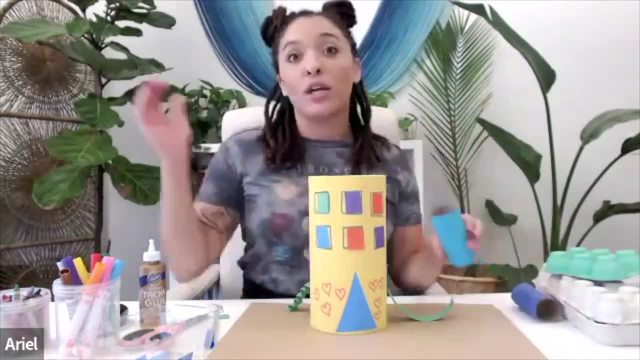 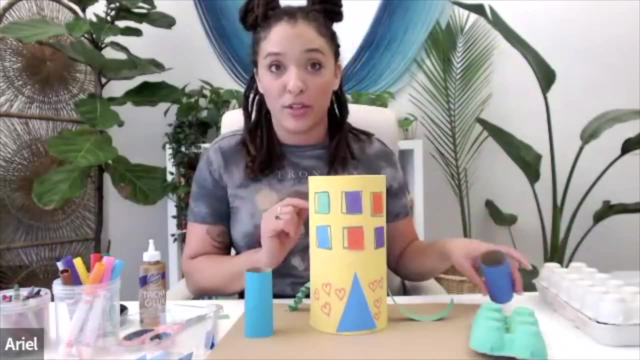 in our video with you today. But remember, you can always keep working on things. Someone right now is also. they told me all the colors they're using and I'm using some of the same colors. They're using red, blue, yellow and green. 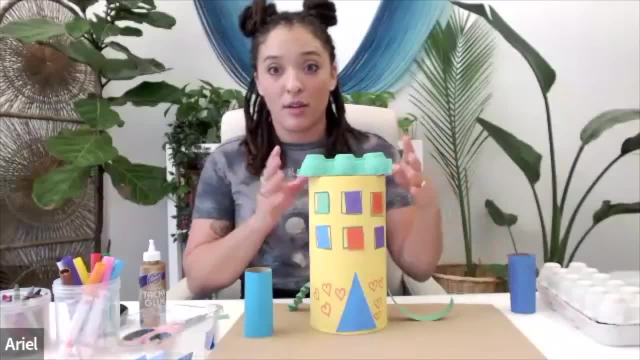 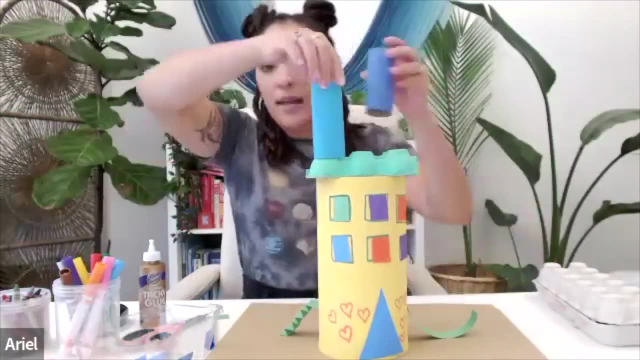 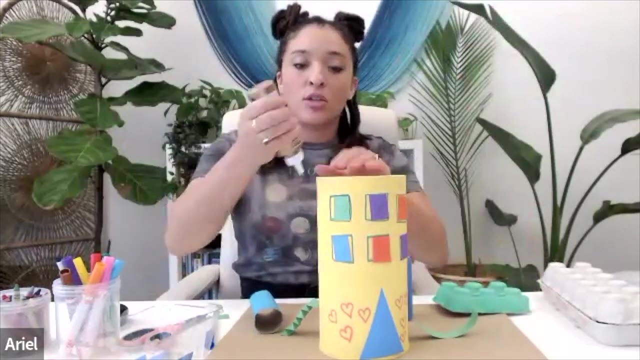 Great combination of colors. Now I'm going to glue this on top of here, and then I want to glue this on top of here and this on top of here, like that. So that's something that I think is a good step to do. 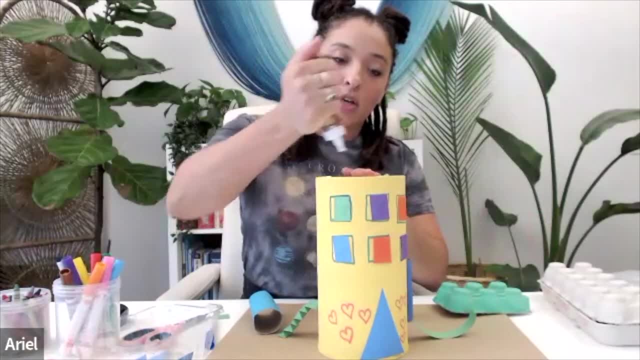 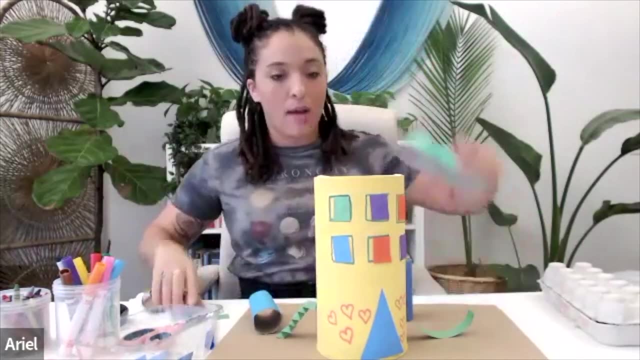 like kind of last is deciding how to arrange it, just because then you can like really work on each piece more easily. You can pick it up, Because once you attach it it's kind of can kind of get a little bit stuck. 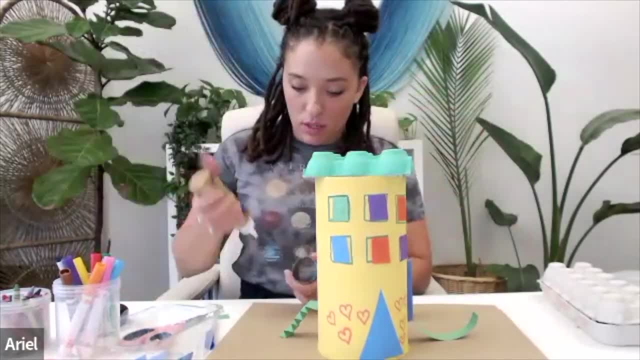 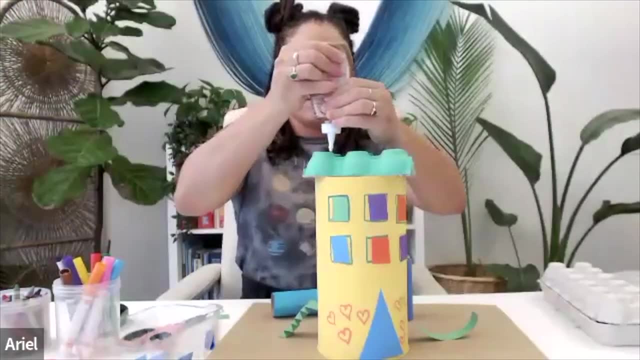 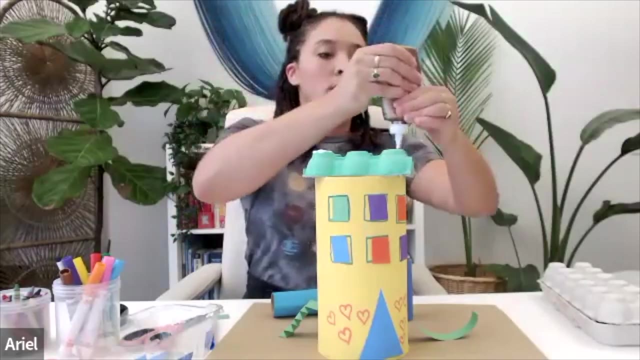 and you want to make sure you can move it around if you need to. Okay, let me try and Okay, this glue is I'm using. It might be coming down to its last bits, but I'm putting some glue in one spot and another spot. 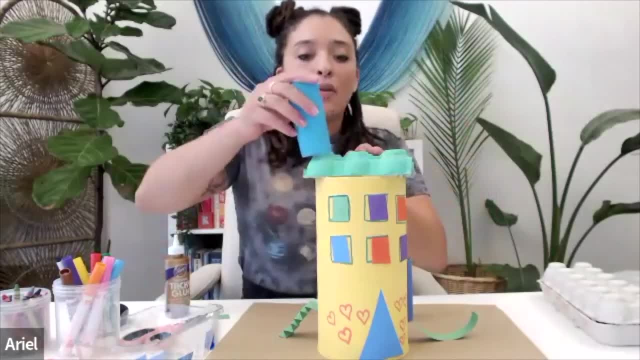 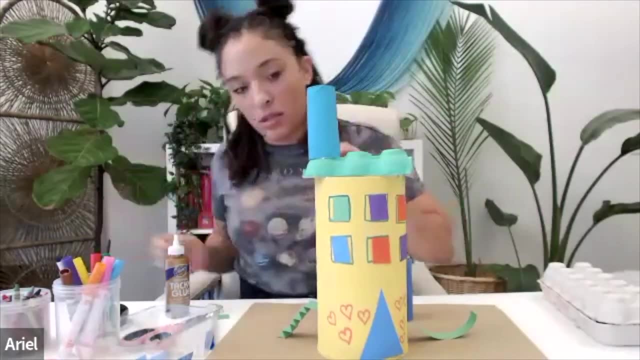 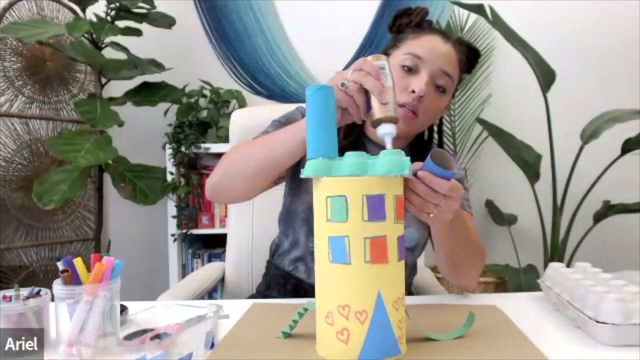 There we go. I really was inspired by King Gilles. He had a lot of towers. Okay, hopefully mine's going to stay. He had a lot of towers in his buildings and so I wanted to. I wanted to make mine. Someone mentioned earlier that they were thinking. 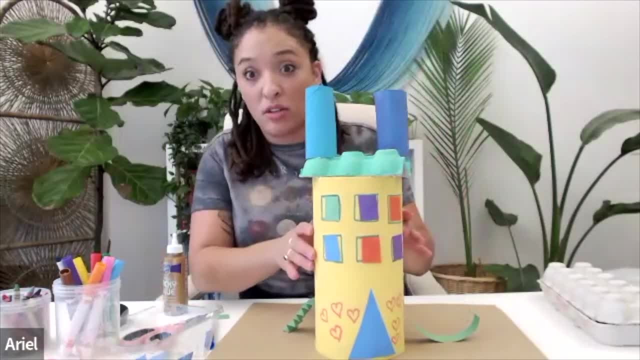 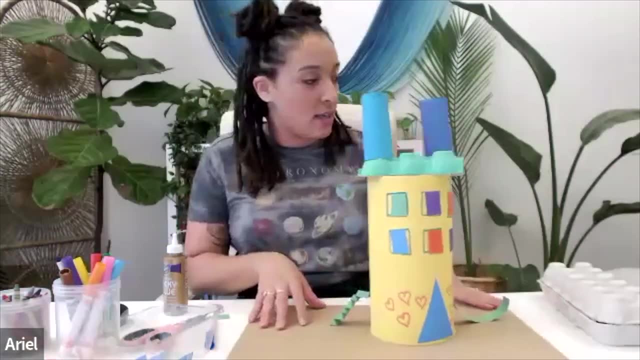 of the Leaning Tower of Pisa. I feel like mine's about to start looking like that too, because I Until this glue dries. it's going to be. It's a little more prone to leaning, so I'm leaning. 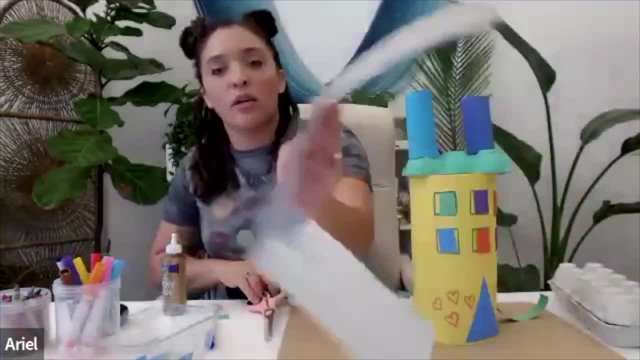 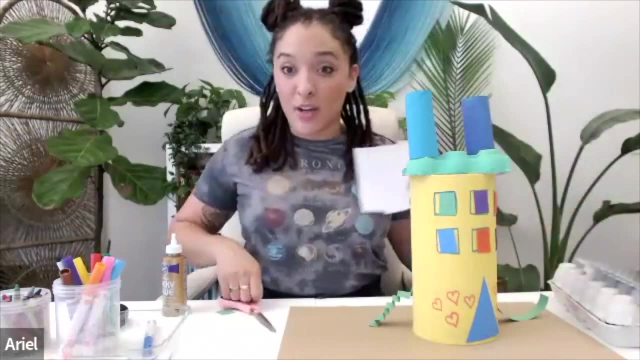 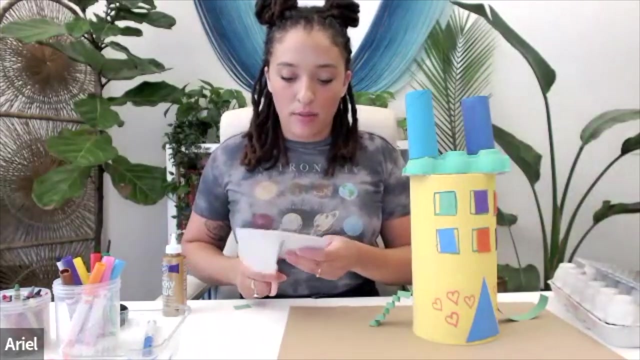 Okay, one more thing I wanted to add. Look at this. I have this like foil kind of paper and I was thinking, if I cut it up I can add a little bit of some decorations at the top of my tower. 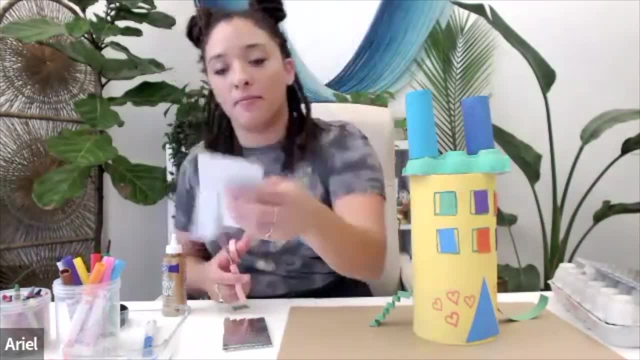 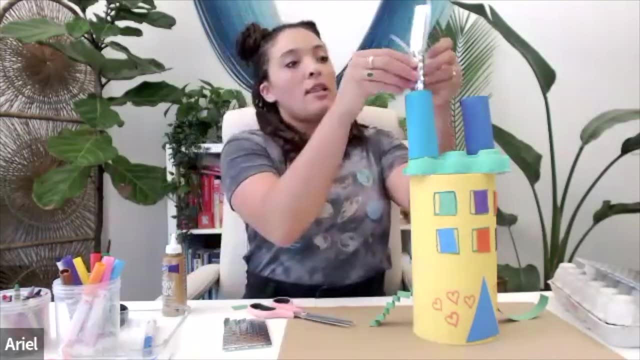 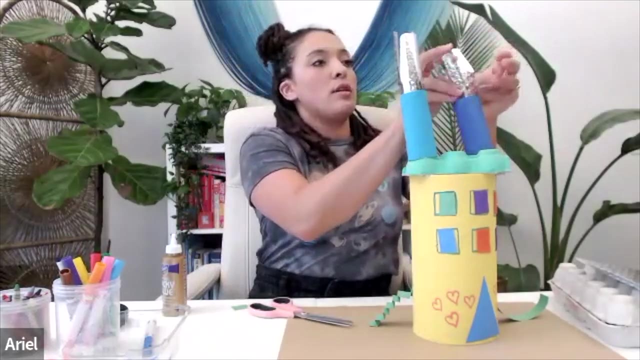 So what I'm doing is cutting it with these little pieces like that. Okay, so they're all little pieces, and then I'm going to stuff them inside of my tower. How do you think that looks? I think that looks pretty creative, right there. 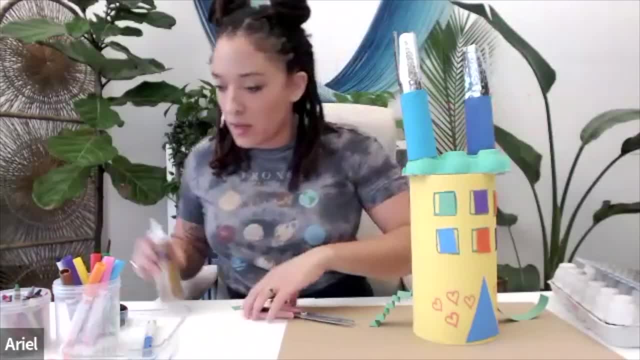 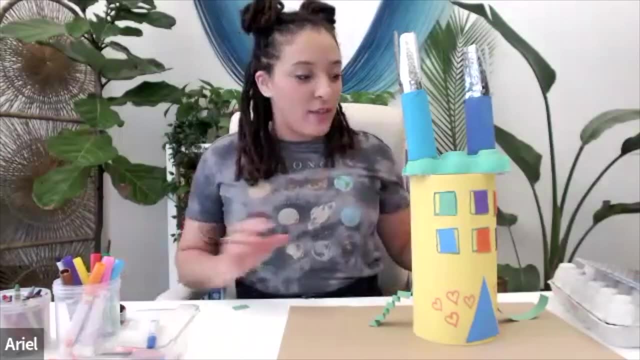 Oh, no See, There's the Leaning Tower of Pisa style. All right. So, friends, this has been really, really fun creating with you all today. I'm sure that you all are doing a lot on your side of the screen.